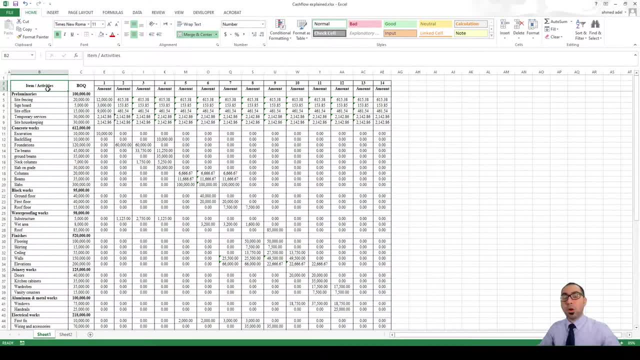 the cash flow. but in order to see the cash flow, in order to do the cash flow, we need first the activities of the project, which will be taken from the items of the BOQ. this is where you get your activity list and before I proceed further, I just want to explain one part here, the first part. 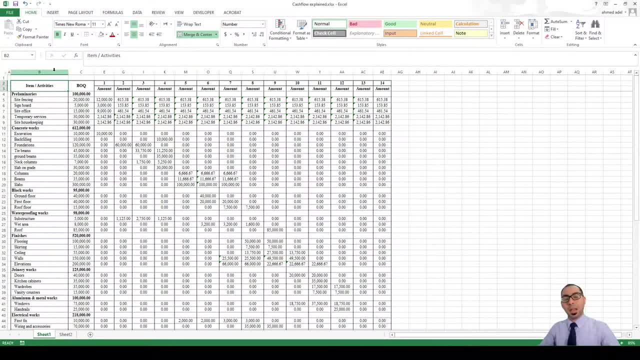 guys in any project is that you will do a quantity, take off okay and prepare a BOQ for all the items with all the quantities ready for pricing. this is the first part and the second part. you will do the cost estimation and you will go into the details of. 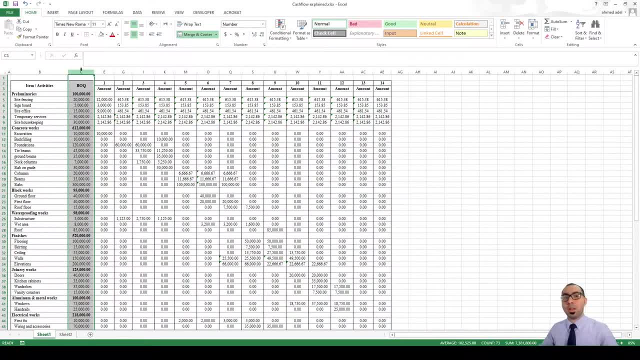 the manpower, materials, equipment, subcontractor and all these things, and when you get the cost of the project you will add the margins to that. then you get your final price, BOQ. I'll leave in the description down below two links for our two courses. the first course: 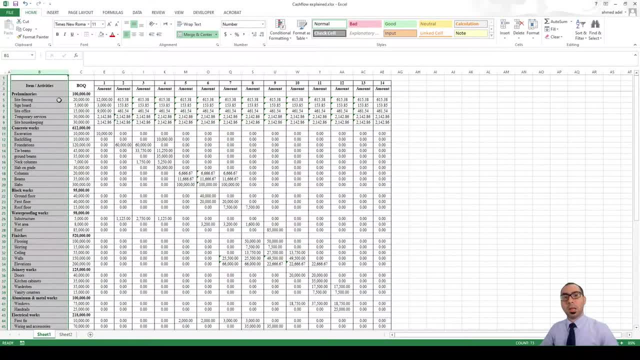 will teach you how to quantify a project and how to make a BOQ, how to study the drawings, how to do the scope of work review and how to keep each and every item in the BOQ. and our second course is regarding the cost estimation, and it will show you in details. 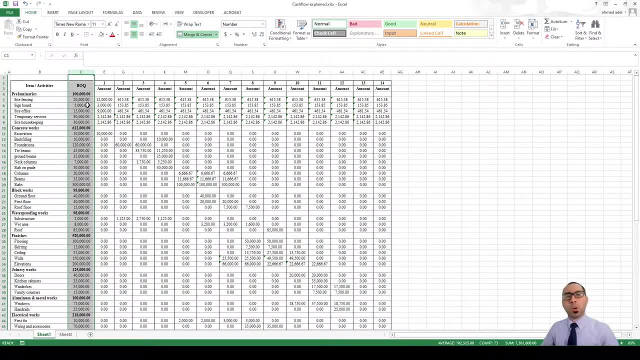 what are the cost elements and how do we like price or estimate the cost of each and every item in the BOQ and then add the margins to the cost that we have calculated in order to get these. so I'm assuming here now that I have a price BOQ where I have all the items and I have all the 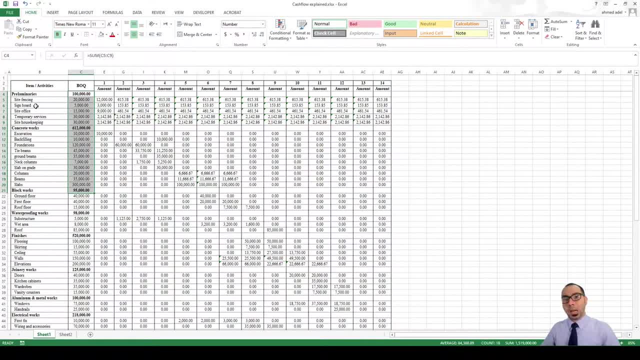 amounts, but this BOQ is like a high level. it is not a very detailed BOQ like I've kept some items here, or the major items, only just for the purpose of this video. there is an important part that I want to discuss here, guys, which is the difference between cost and the price. these are very important. 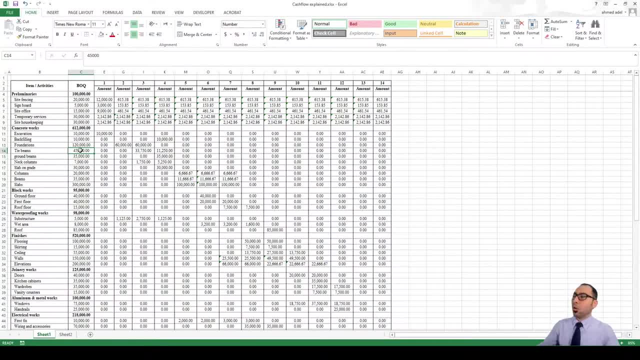 I told you that it depends on the cost. yes, I asked about the cost of the Admiral, really. but one more thing about this: BOQ is exactly the same: the difference between the cost and the price, and the cost is not the cost for me. this is my content now. then let me try this slow 것 and 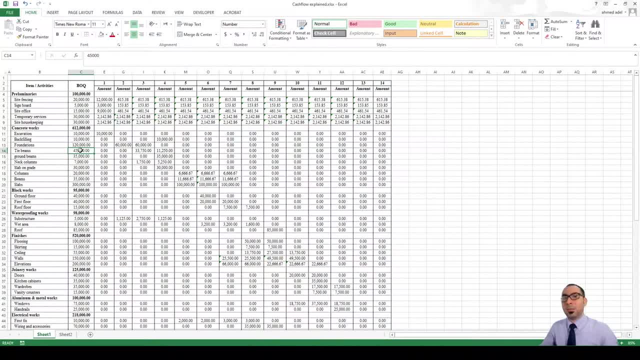 all the examples so I shouldn't be wasting my time while editing. I just want to give you an idea of the scenario. but let's assume that the cash flow is mature. let's assume that this is a good requirements. he will put it on the drawings and then he will give me my drawings for the project. 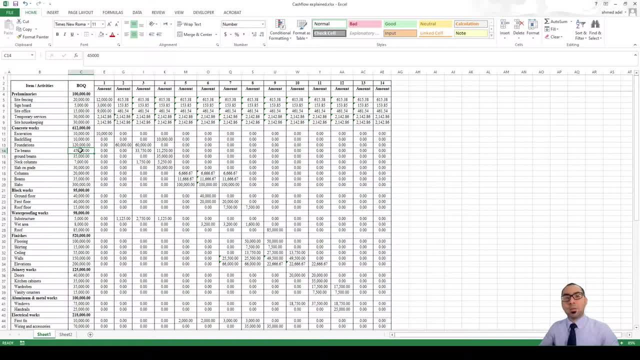 or for the house that i want to build, and i will give these drawings to a contractor in order to price it for me. because how do i build the house? i need to hire a contractor, so i'll make a tender, or i'll just go to someone whom i know- a contractor that i know- and i'll give him the drawings. 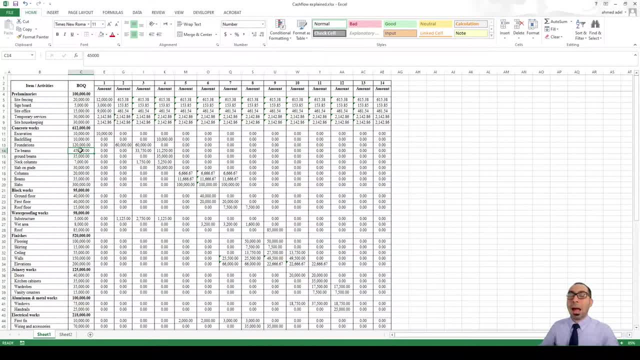 and he will give me his price. now how he will give me his price: okay, he will do some cost estimation activities in his office. he will do what i told you now: he will calculate, he will make a boq and he will calculate the quantities and then he will estimate the cost. 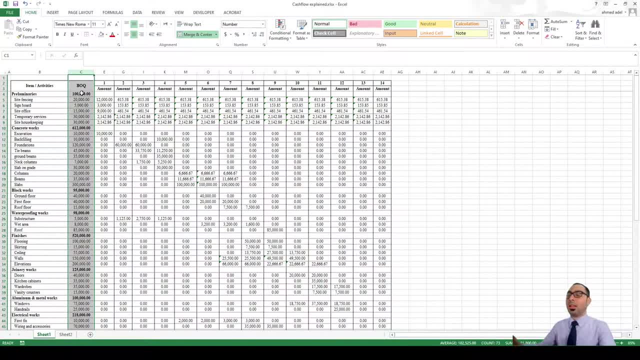 then he will add his margins to his cost and he will give me his price. so from the point of view of that contractor, okay, he did his cost, he understood how much these works will cost him and he added the margins that he wants on top of this cost. 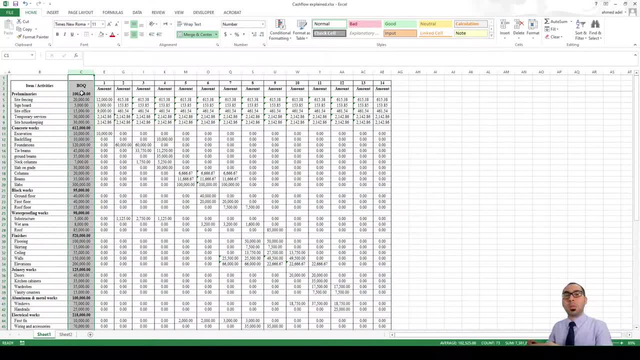 to the estimated cost and this becomes his price. so he gives me his price. so his price is his cost plus his margins. okay, but my cost as a client, as a house owner, as the one who wants to build a home, as the happy man who wants to build a home, this will be my cost. okay, guys. 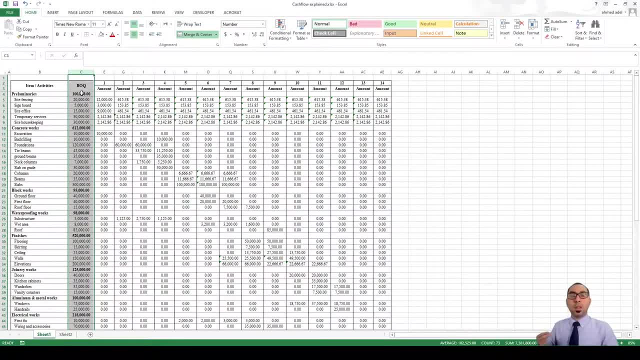 so my cost as a client will be the price of the contract. i'll say it another way: consider me the contractor. okay, if i am a contractor and someone gives me the drawings to give him my price to execute this job, what i will do, i will quantify and i will price or or estimate the cost. then i'll. 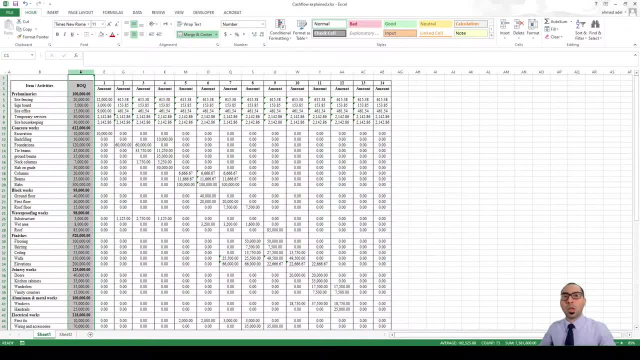 add the margin, then i'll understand how much is my price to execute these works and i'll give him my price, my cost plus my cost margins. good, and for him, for the client, this will be the cost. okay, guys, his cost is my price to build his house. so what i want to say now is that this is the price that i am going to give to my client. 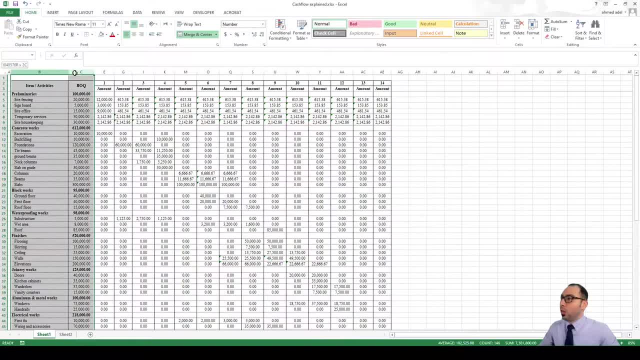 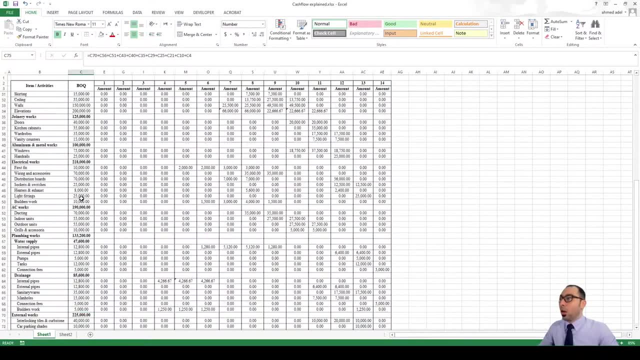 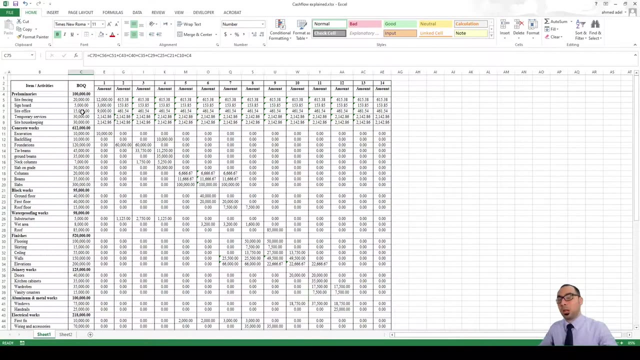 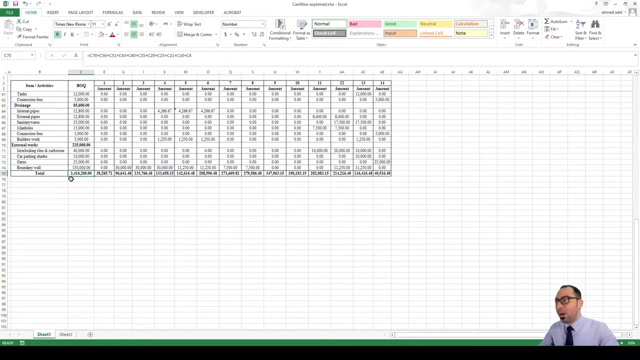 okay, so our price to execute this project is this much here: 2.416 million. okay, so this is the boq. that includes my costs and it includes my margins as well. so this is the boq that i am going to give to my client- and he will, if he likes, my final price. 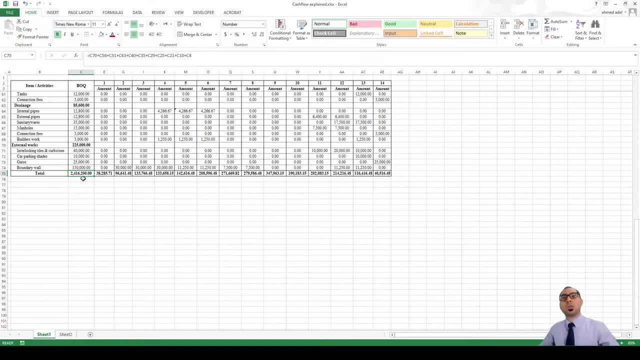 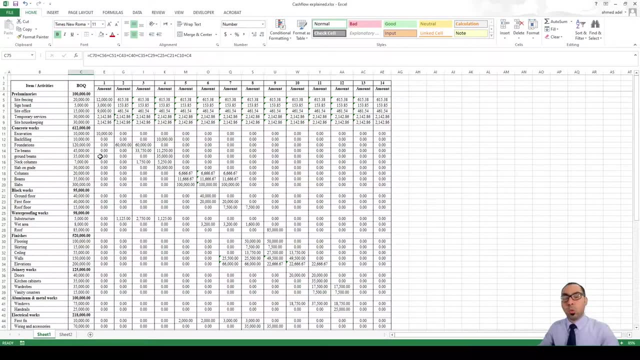 he will accept me as his contractor and i will start doing the work. okay, so the first part that i i'll do when, when i get a new project, the first thing in the first one or two weeks or 10 days or whatever, i have to submit my program of war. okay, my detailed program of war. and what is that? 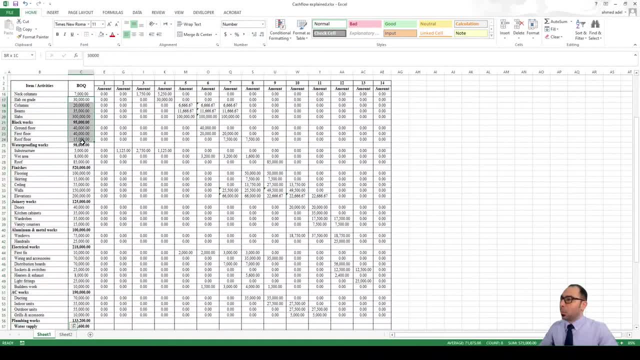 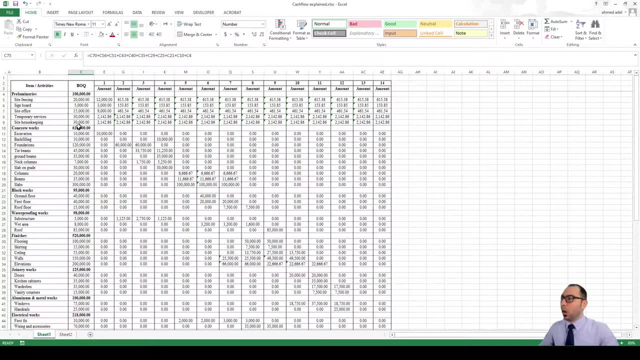 these are the items of the boq and these are the prices of these items and this is the total amount. okay, i need to give him a program when i will do what. this is the time schedule, guys, or the program where you will schedule all these items or all these activities, which is the project. 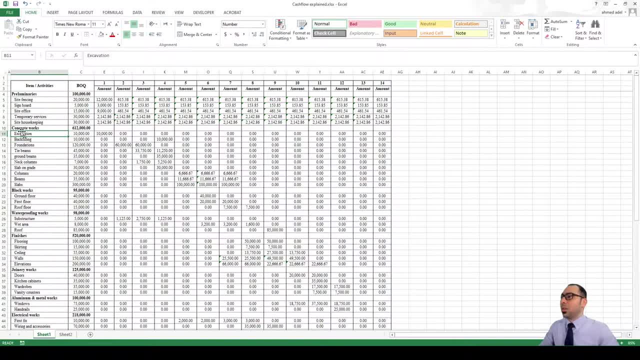 actually okay, like, for example, the excavation. we know that the excavation will cost, will cost the client 10 000 because my price for the excavation is 10 000. but how much is my cost for the excavation? no one knows, or only i know. okay, my client doesn't know that. my client have 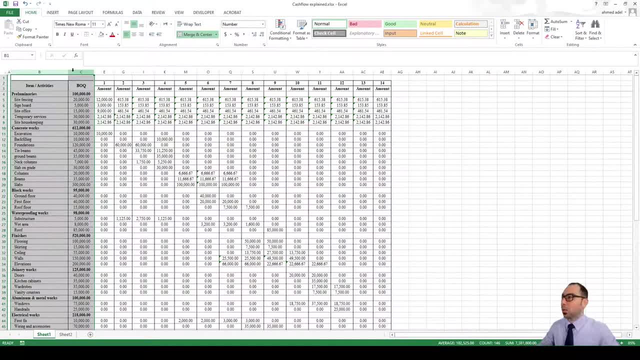 his boq here that i gave to him, which is my price. so, if i am assuming, i will make a program now and i will say that the excavation works that worth 10 000 will be executed in the month number one of the project. okay, let's take another example: the slab on grade here. that will cost the client 30 000. 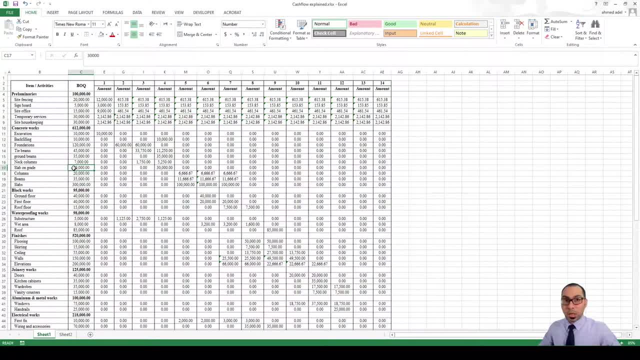 this will be executed as per the program that i will give to my client in the month number four. now the third course will be how to make a program, primavera p6- that shows you each of these activities, when is the start date and when is the end date, okay for this particular activity, and from the boq you have the price of this item. 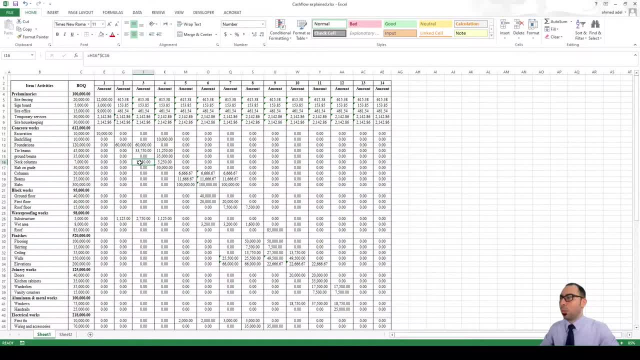 okay, nick columns, for example. here we are assuming that part of the nick of the nick columns will be executed in month number three and another part will be executed in part number four. so this 7 000 part of it will be required from the client to me in month number three and another part is required. 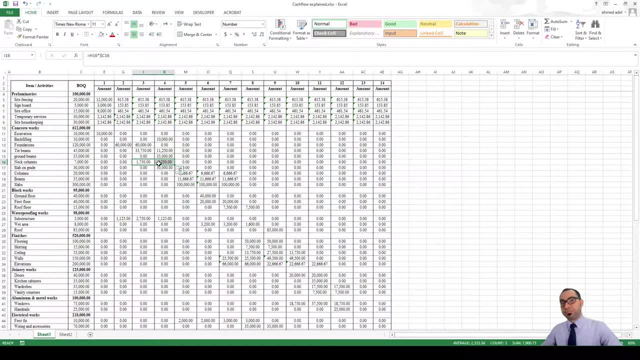 from the client to me in month number four. but the scheduling itself is what you need to learn here. you need to know how to create this program and after you create the program in terms of durations of the activities and the relationships between these activities and the total duration and everything, you will submit this program to the project. 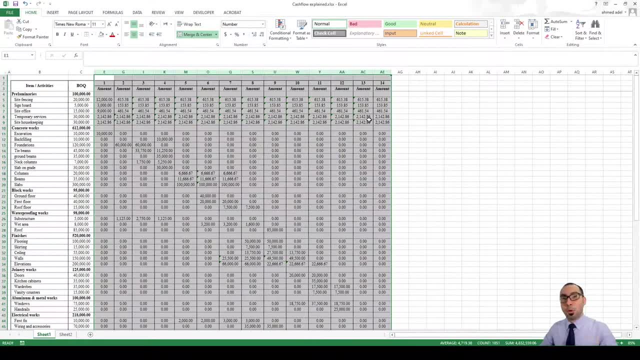 engineer or the project consultant, if he approves your methodology, that that the way that you will execute the works. in that case, you will take this approved baseline program and you will start loading the costs of the boq items on the project activities. the example that i i showed you now. 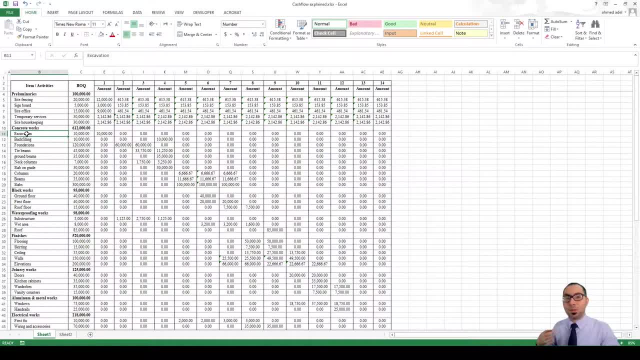 which is excavation. the excavation is scheduled for for me in my program to end to end by the end of the first month, so i'll execute excavation in the first month, by the end of first month. anything that has a value here should be completed. like in the first month i'll do the site fencing. 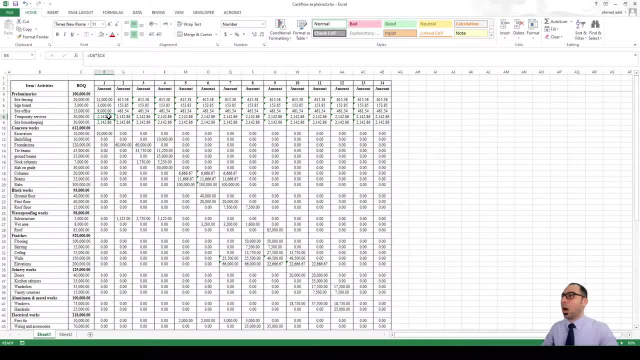 i'll put the sign board, i'll put the site office, i'll put i'll apply, for example, or i'll pay for the first bill of the temporary- uh, temporary services. i'll do the first site housekeeping, okay, and so on. what are the activities that i have scheduled in the upcoming month and how much? 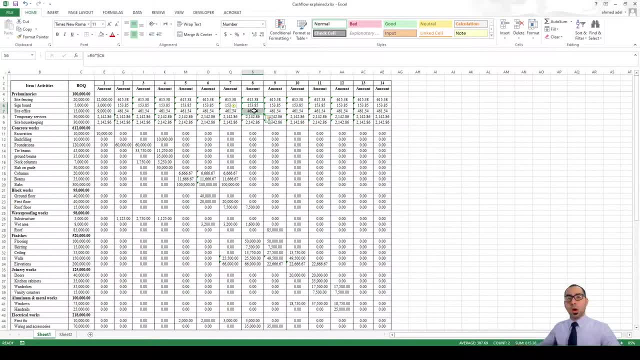 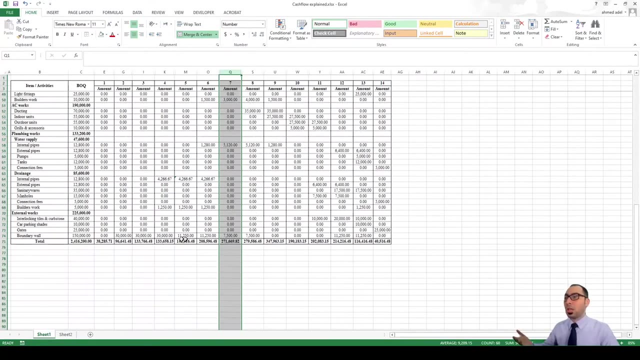 is their costs. so we will do a program and we will load the boq costs on the program. when we do that, guys, since in the program we know what are the works that we will be doing in each of this month, we know how much is the cost of the activities or the items that will be done, or? 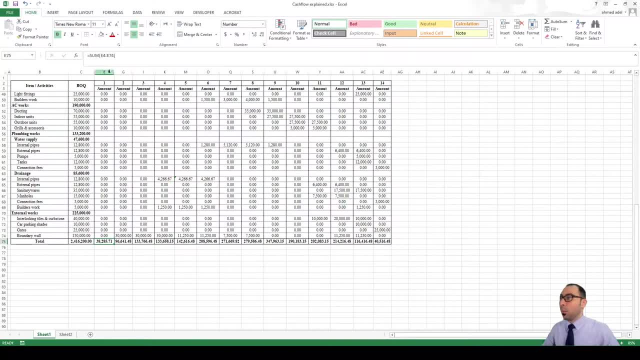 completed in this month. so simply by the end of the first month, if i follow my program, i will submit a bill to my client that is 38 285.71 currency, whatever currency, this will be my bill that i will submit by the end of that month, because 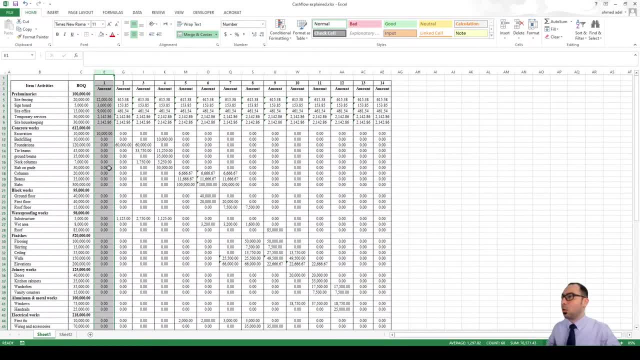 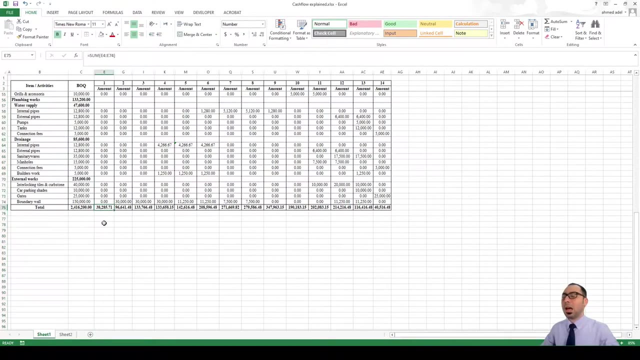 my assumption, my plan is to execute these items in the first month. so what is the value of these items? as per the boq, these are the values and this is the submission by the end of the first month. okay, this is the value of works completed by the end of the second month. this is the value. 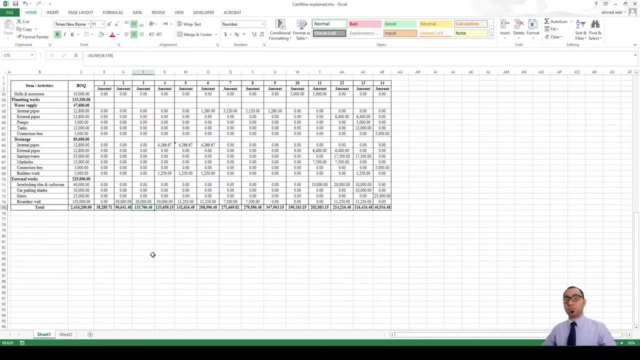 by the end of the third month. this is the value. so now i have the duration, which is 14 months, and i know this total price- my price total 2.4 million- how the client is going to pay this amount to me. okay, he will not come in the first day and say: 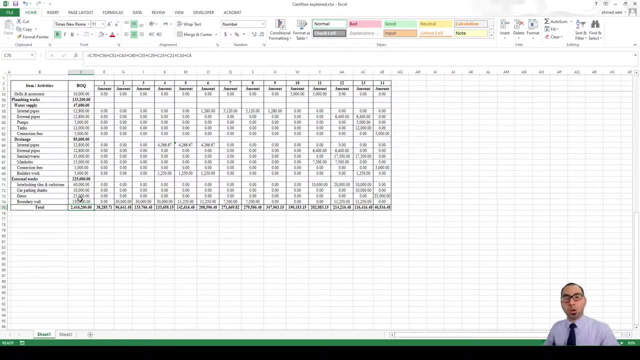 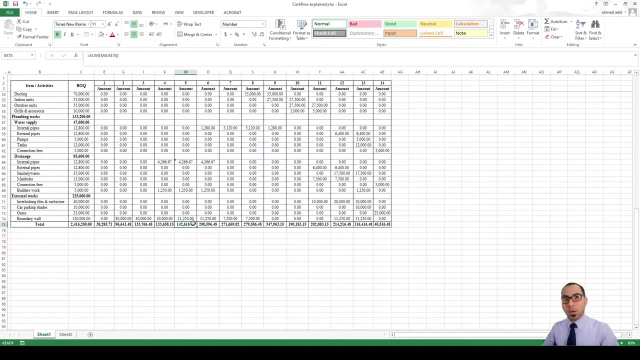 all right, take 2.4 million and go execute the works. no, it is not like that. it depends on the works that i will execute in the first, second, third and so on. and we understood how these numbers are calculated or where they are coming from. okay, so what we have done so far is that 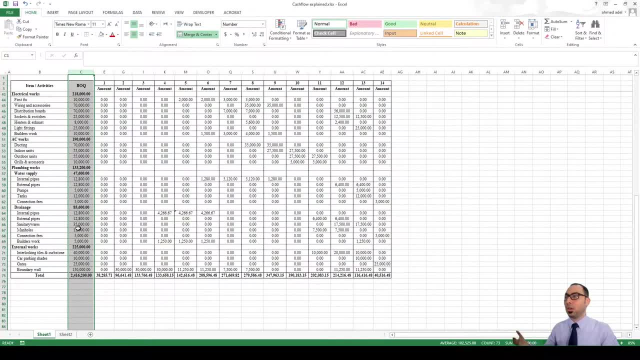 we have made a program and we have loaded the costs on the program, so we got something that we call the cash flow or the cost baseline. okay, and the cost baseline or the cash flow is a time phased cost. time phased cost means what means that this project will cost, will cost the client. 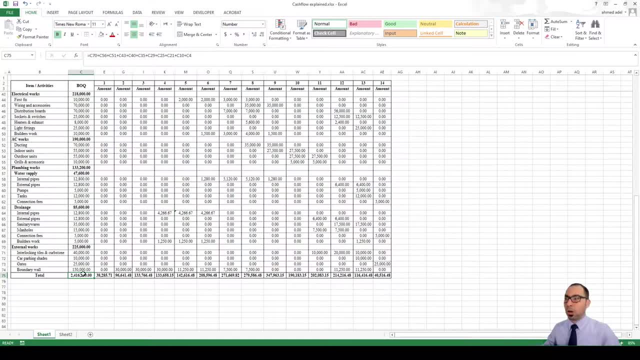 in the end 2.4, because my price as a contractor is 2.4 but, as we said, it is not in the first day 2.4. no, he will pay the 2.4 over 14 months and this is the plan, how he is going to pay the 2.4. 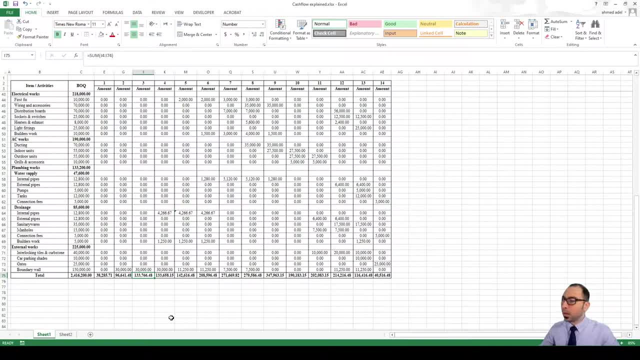 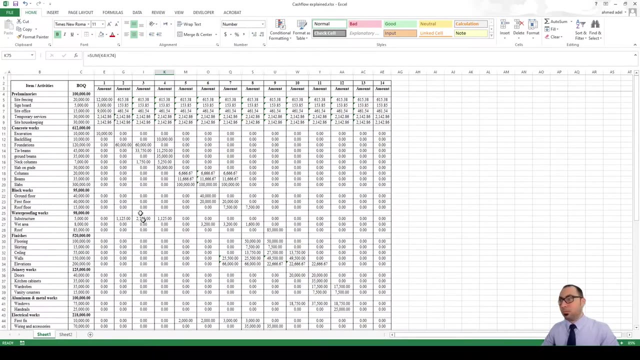 how much he is going to pay every month. so what we have done here, guys, is called the planned values. these are the planned values. why these are the planned values? because we have the planned values. these are the planned values. because we have the planned values. the planned values because, as per my plan, i will execute the the project as per this scheduling for. 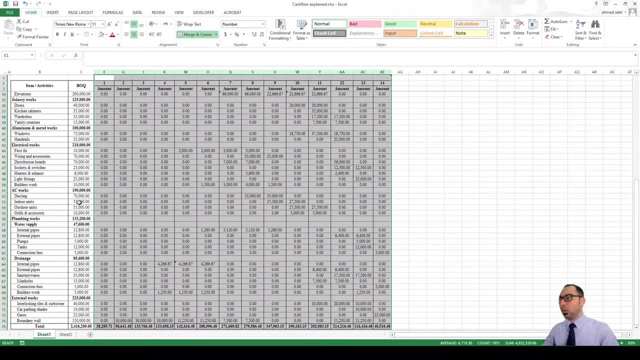 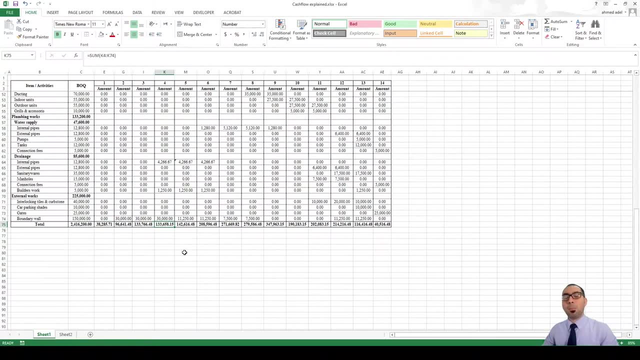 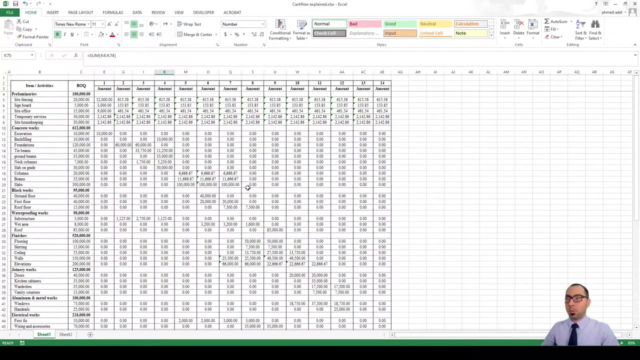 the various activities and when i loaded my price on these items, i got this cash flow, which is the plan. these are the planned values. so what's next now? i believe, guys, we understand this part and we understand that if you want to know how to do the boq, we have a course for that link in the 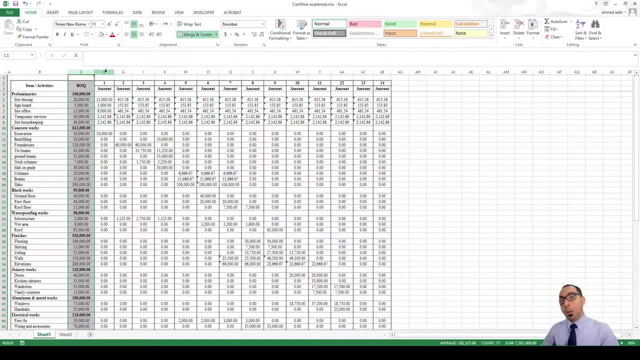 description- cost estimation link in the description. the upcoming one, or the course that we are working on now, is planning and scheduling, and this will include preparation of the program and loading the cost on the program as well. this will be our course number three. okay, what happens after that? 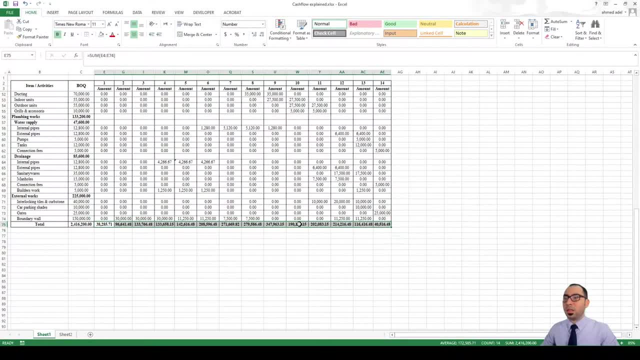 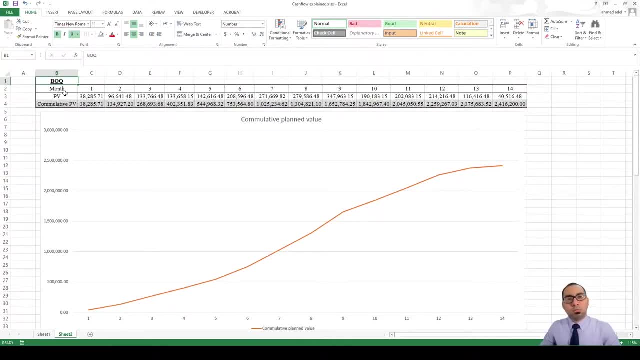 our boq is our price as a contractor to execute this job. we have done a program of works or we have scheduled the activities and from our plan, when we loaded the cost on our plan, we got something called the planned value, which i just showed you, these numbers here. 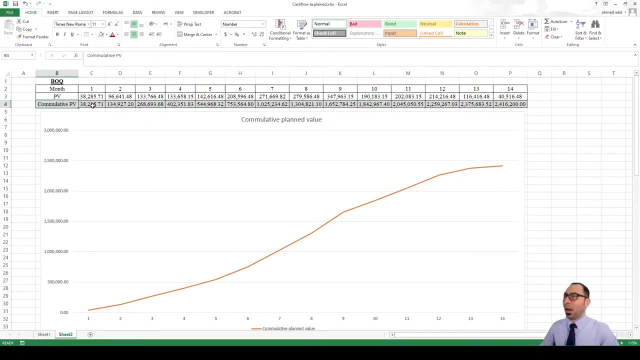 and when you go and take the cumulative planned value- the first one here will be equal to this- then the value by the end of the second month: how much is your plan cumulative planned value by the end of the second month? it will be what you have finished so far, which. 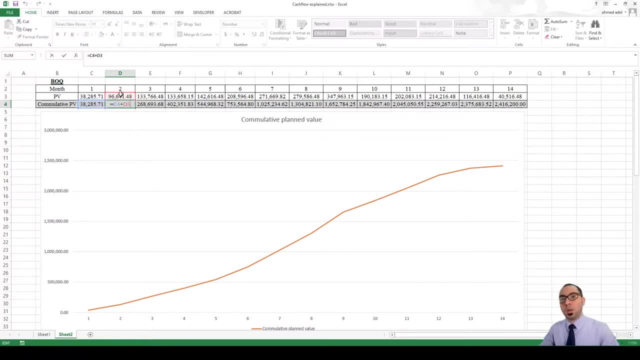 is only the first month value plus what you have finished in the second month, and the cumulative planned value in month number three will be again what you have completed so far, which is the planned value of month number one plus the planned value of months number two plus what you have completed in the month number three. so 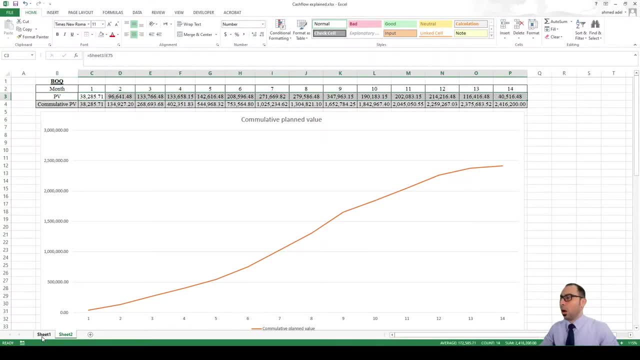 basically the planned values here. are these values okay? and the cumulative is just the first. one is equal to the first one here. second is this plus this, third, this plus this for this plus this. so basically it's equal to what you have completed so far plus what you have completed this month as well. so, by the 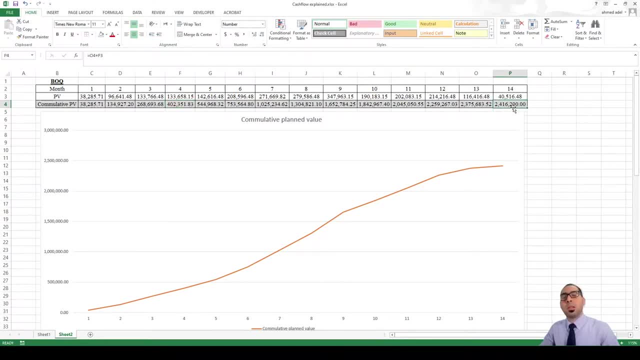 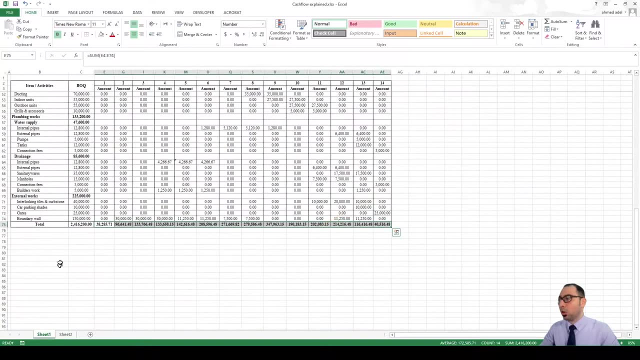 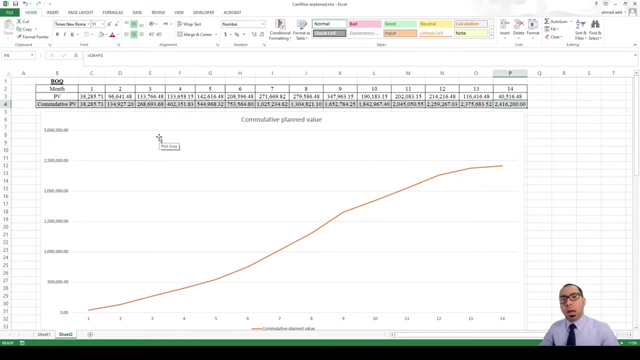 end of the 14th month, you would have completed the fully scope, which is the full bill. you, which is that two point four, one, six million, which is your contract value, which is your price for this project. okay, so when you go now and you draw the relationship between the month, okay, month number. 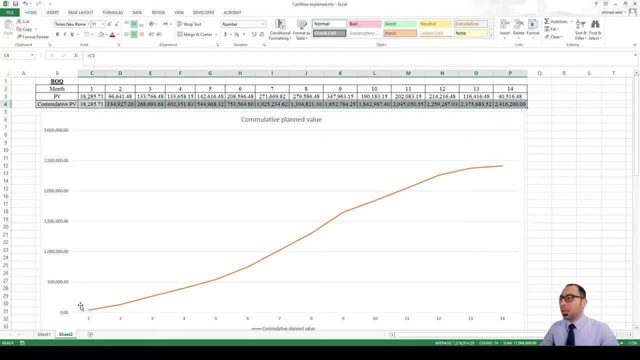 and the cumulative planned value, you get something that looks like that: okay, guys, this is the s curve, or this is the cash flow, this is the cost baseline, this is the cumulative planned value against the month number. call it whatever you want, guys, but now we understand the concept that. 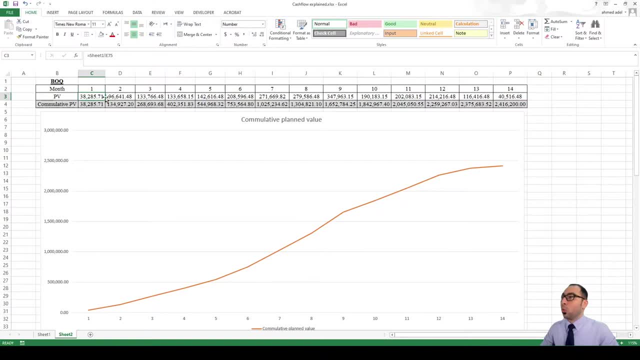 month number one: i'll do works that worth 38 000. month number two: i'll do works that. this is my plan, guys, these are the planned values i am. i didn't do anything yet. i just prepared the program and i loaded the costs. so this is my plan. i am planning i'll do it this way, but how actually? i? 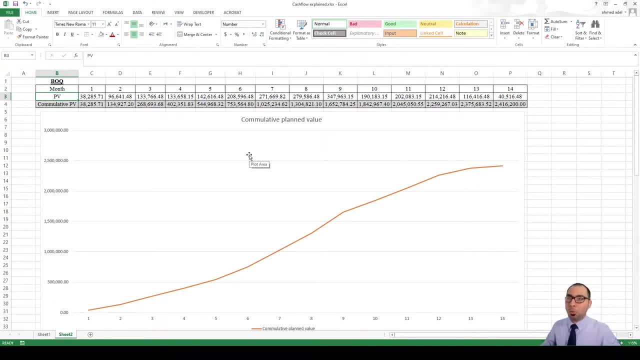 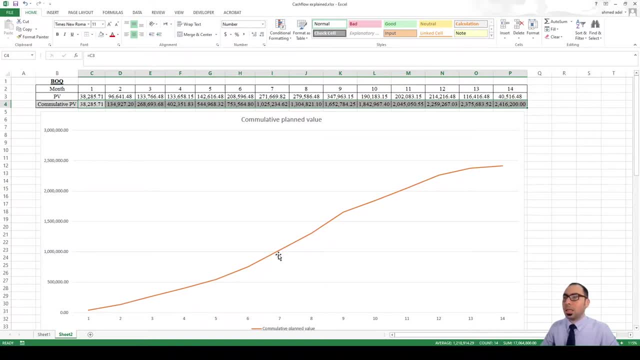 get this look okay. so it's increasing, increasing and here because, like, let's say, from month number four to month number 10 or 11, you will be doing the majority of the works. so that's why it's going up very fast here, because, as per your plan, let's go back to our plan here. you see, guys? 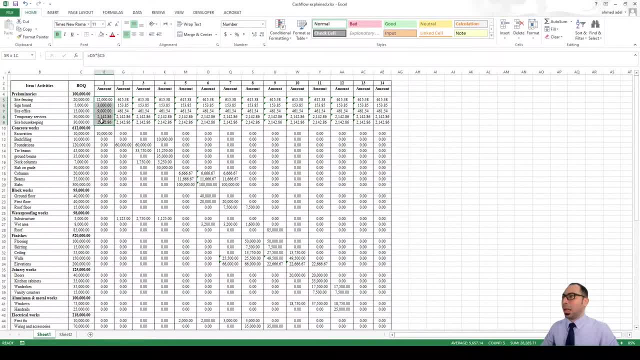 you see guys, you see guys, prelims. i'm assuming that i'll do the establishment only then. these are running costs of the prelims: excavation, for example. i am doing it in the first month, then second month. what i'll do? i'll run my prelims and i'll do the foundations, and here i'll do also the waterproofing for foundations. nothing. 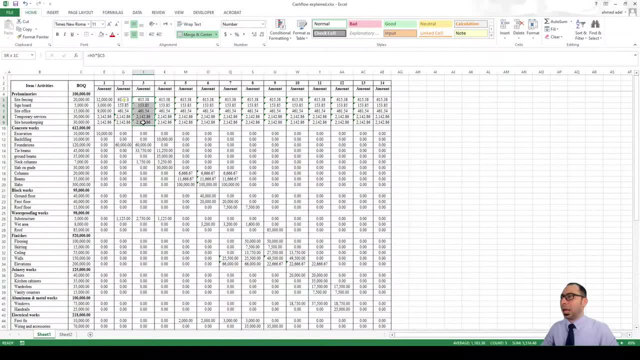 more. okay, like let's go to month number three. again, i am running my prelims and i'll execute the remaining part of the foundations, and then i'll do the foundations, and then i'll do the And I'll do also the tie beams and part of the neck columns. 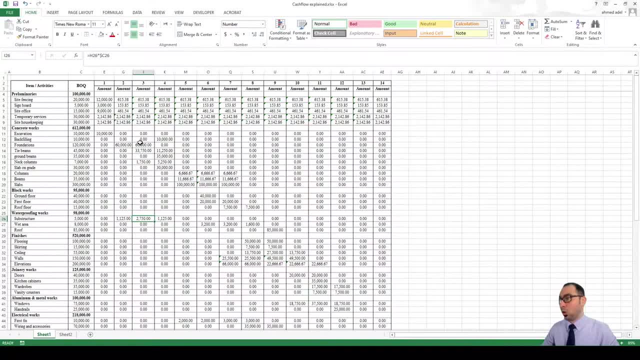 And I'll also do a part of the waterproofing works, because these elements need waterproofing And what else Nothing. Month number three: we are assuming here that we will- sorry month number I got lost, guys. Okay, anyway. month number four: I'll do the back filling. 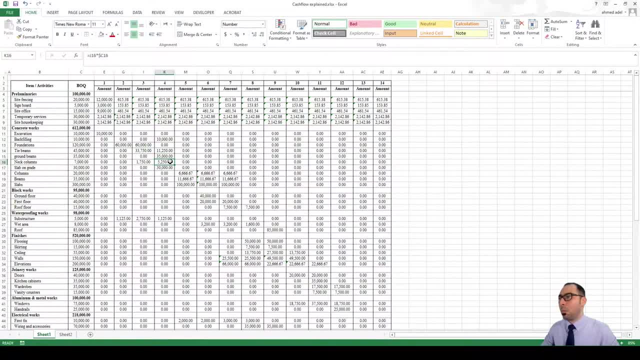 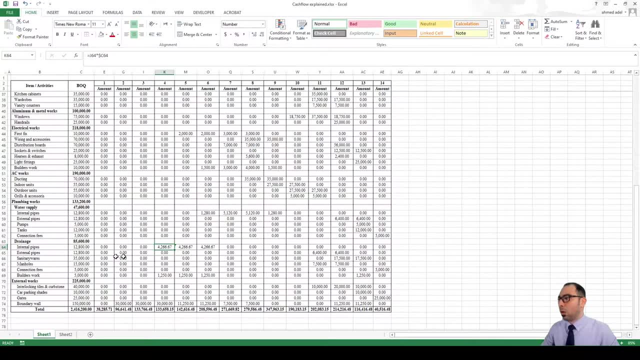 I'll do the tie beams, I'll do the ground beams, I'll do the remaining part of the neck columns- slab on grade and again some parts of the waterproofing. And here I'll do some drainage pipes below the slab on grade and some builder's work. 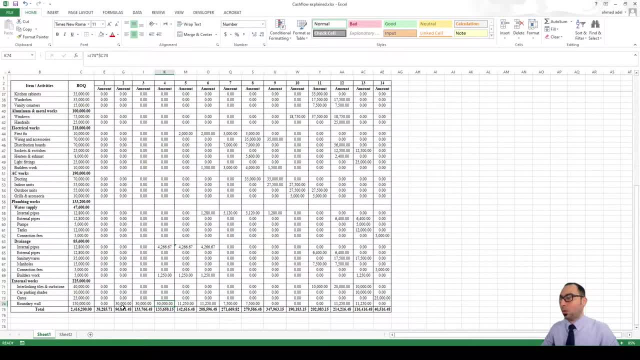 will be there for that, And I'll do also parts of the boundary wall here in the first and second, third and fourth months and so on. So as per my program, what I am going to do in which month we are doing the scheduling. 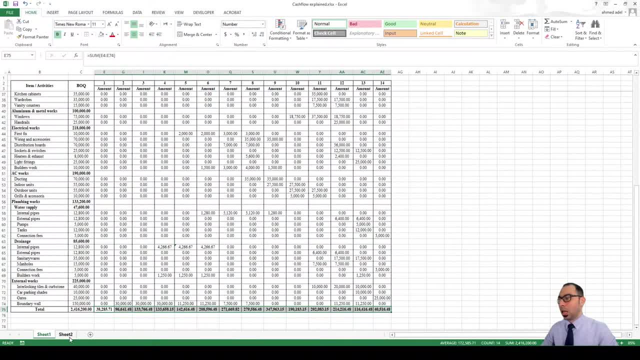 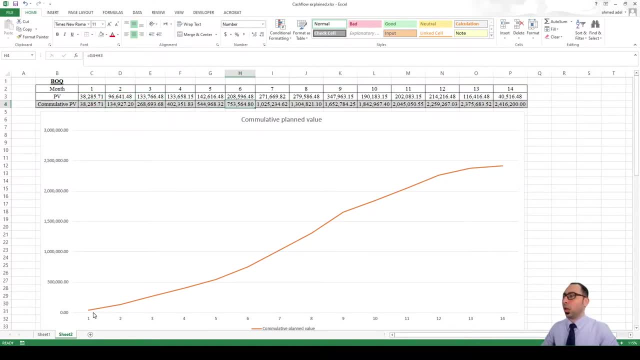 and we load the costs to get these numbers and then planned value each month. This is the planned value And this is the cumulative value. And when I draw the relationship between the month number and the cumulative, the cumulative planned value, again I explained why it is planned. because it is as per my plan and my 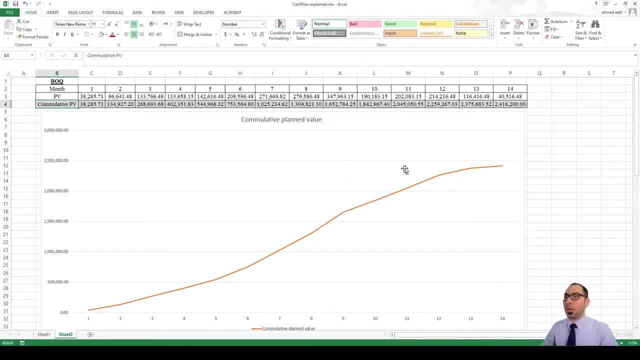 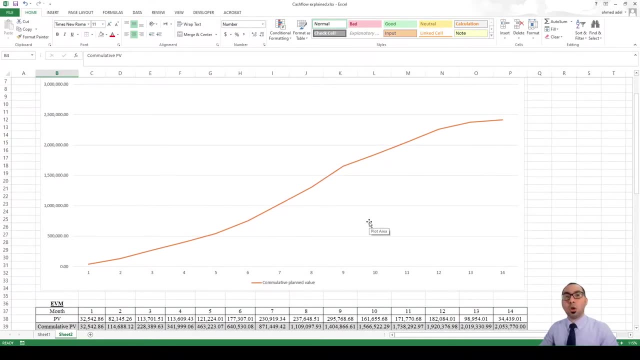 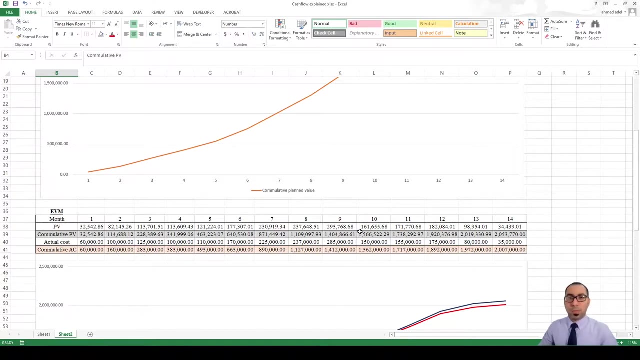 BOQ prices? it looks like that. Okay, so I am getting this Very good. Now, this is our planned cash flow, or our cost baseline. Now, what is that? fourth part, Part Guys, two courses there in the description. one course is under preparation at the time. 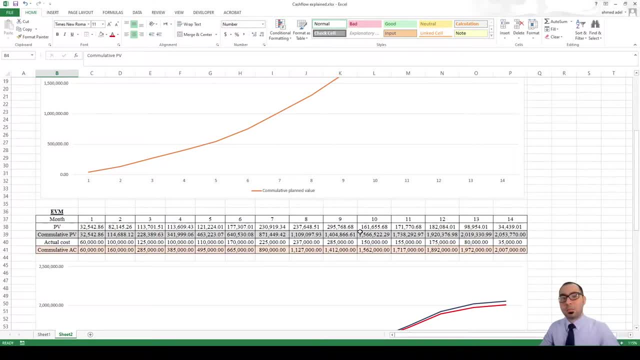 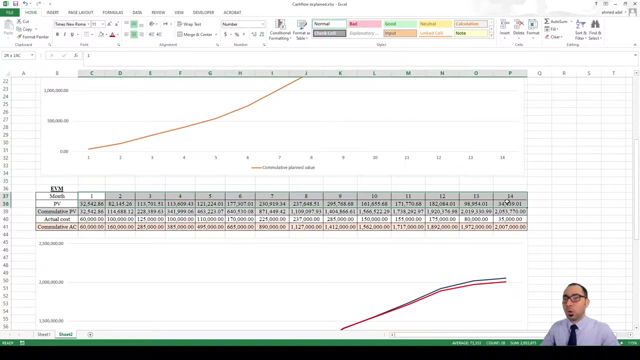 of filming this video. the course that will be after that, the course number four, is cost control, guys, which I am going to explain here now. What is cost control? As we discussed? now we have the month number, Okay, And we have the planned value. 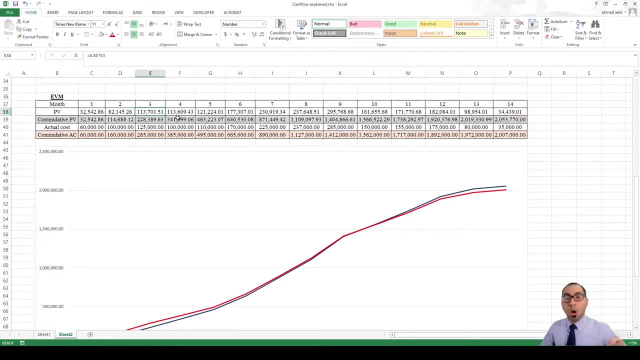 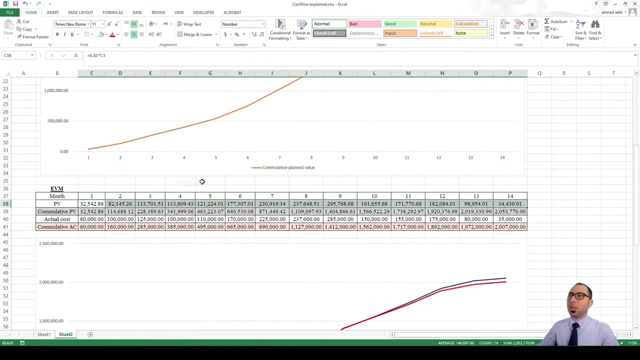 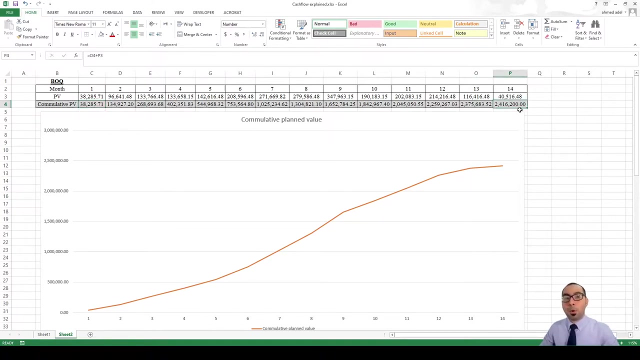 How much is our plan Worth of works every month as per our approved project program or schedule? So these are the planned values that we discussed just now. There is a very important part here, guys. As you can see, the cumulative planned value here is 2.416,, which is the project price. 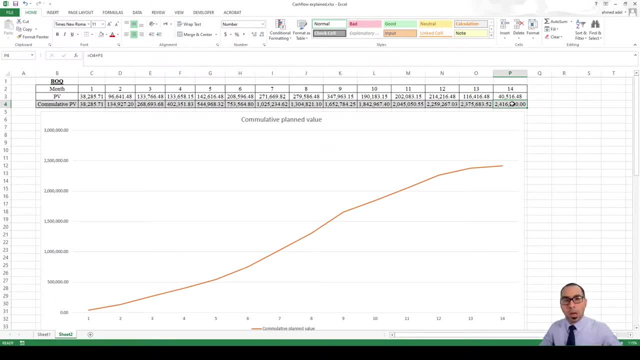 Okay, This is our price that we will give to our client to execute the works And this is the cash flow that we will give him. also, And this will be our approved cash flow that we will give to the client, So he has to prepare himself to pay us these amounts monthly. 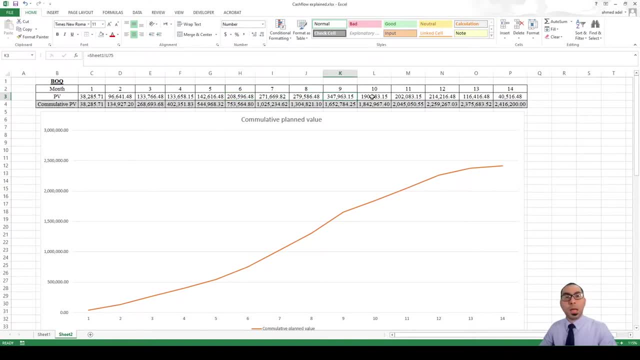 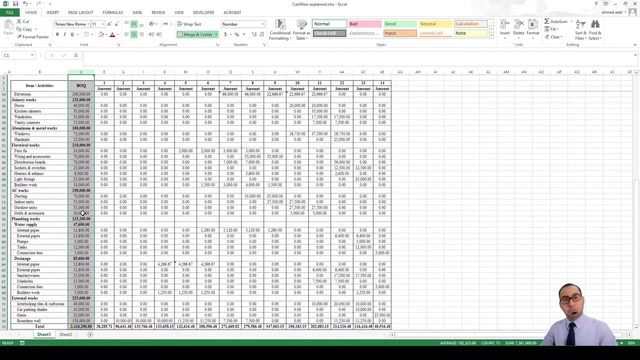 He has to prepare these money, monies, monthly to pay us for the works that we are going to do, because our plan is to execute the works this way. Okay, If this is my price, guys, if these values here, the BOQ, are my price, that doesn't mean that these are my costs as a contractor. 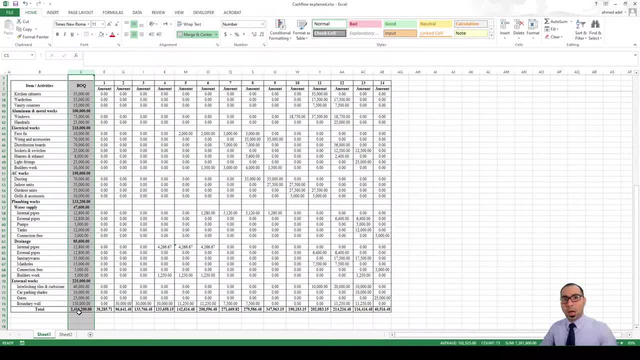 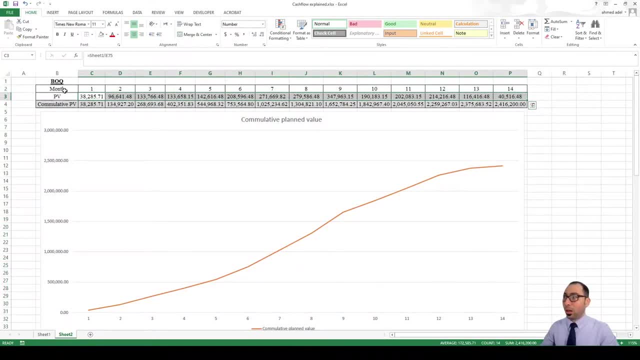 Correct, Because my price that I will give to the client is my cost plus margins. So now what I have done so far is that I have given the price- okay, the cash flow of the project price, But actually I'm not going. 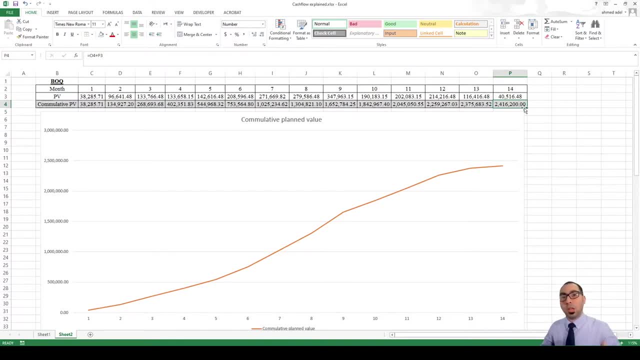 To cost myself 2.4 to deliver the project, to do the works? No, because there are some margins here that are for me, for my company. So we go and prepare something called the project budget, which is almost similar to the cost estimate that I have done for the project. 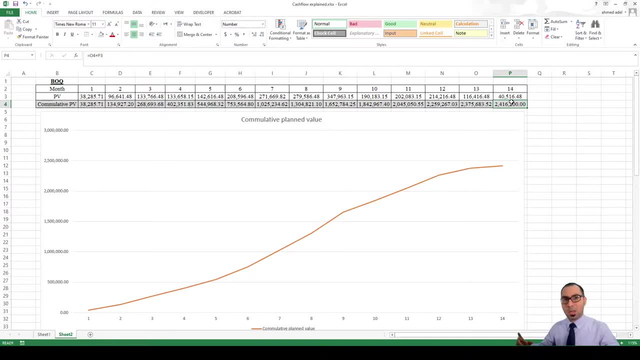 I just remove the margins and whatever cost estimate that I did. this will be my budget, Because when I was pricing this is my budget, When I was estimating the project, when I was estimating the project, I assumed that I will spend this much to execute the works. 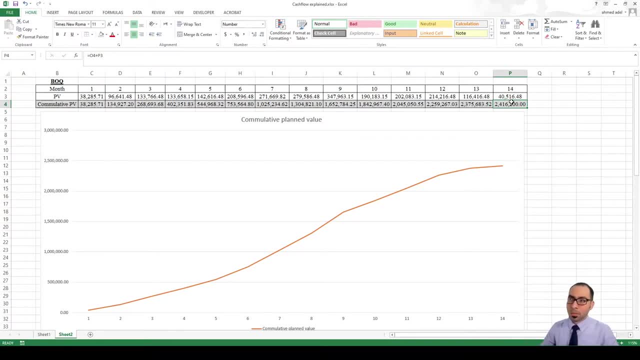 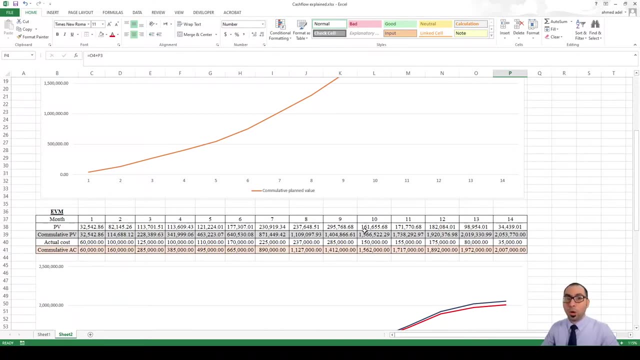 And I added some margins to that. So what I am going to do now here internally, internally inside my company, no one will do that will know that I am doing this. I will prepare a project budget. I will go to my price. 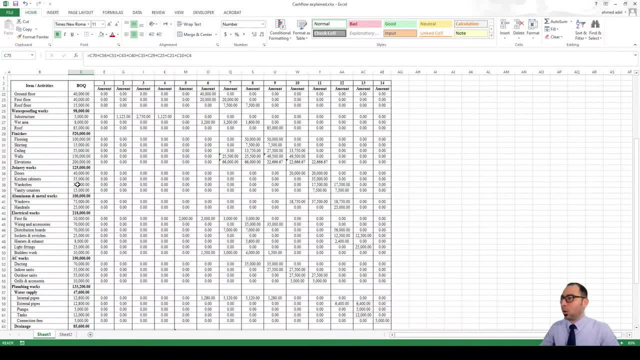 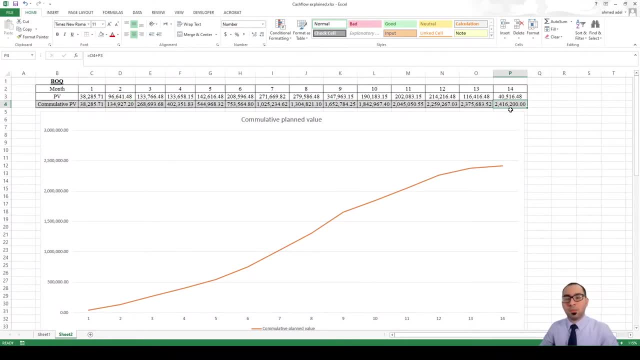 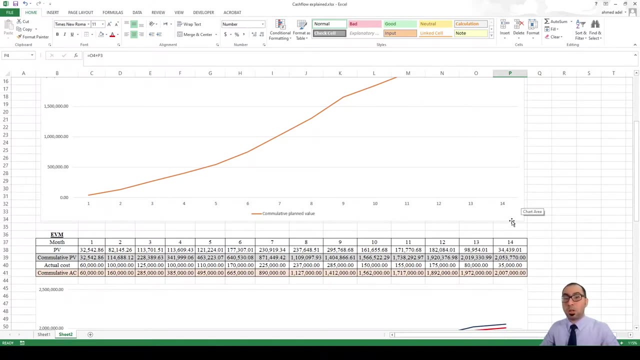 And this is the breakdown of my price, how it is 2.4.. Because these are the Prices. so I will go to my price here and I will start removing the margins, because I want to see my budget, which is my cost estimate or my dry cost, without any margins. 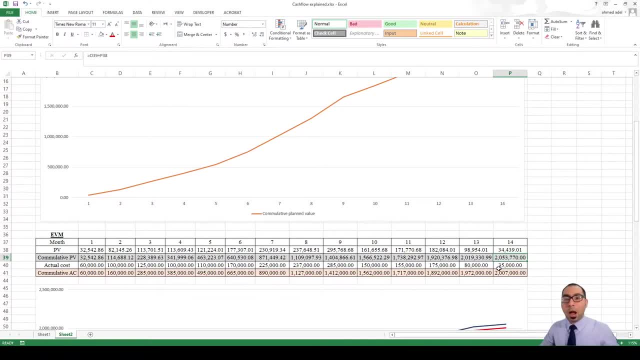 So I am assuming that or my budget I am planning, or I am going to execute this project at two million and fifty three thousand only. OK, because the four hundred thousand are my margins, I am assuming here. So I have prepared a budget, OK, that will be executing, that will result in executing this project at two million and fifty three thousand. 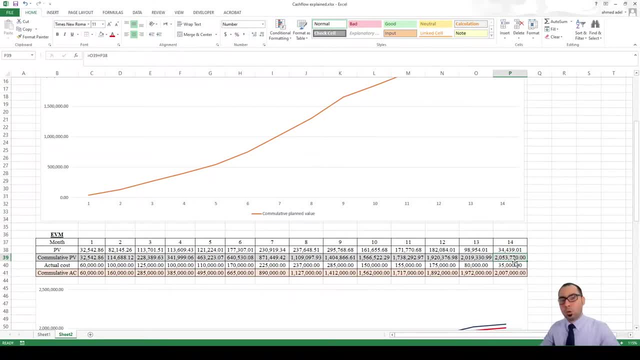 Now the first part that we will do in our course number four, which is the cost control, that we will show you how to prepare this budget. Actually, you have seen the cost estimate, or those of you who have attended our cost estimation course already. 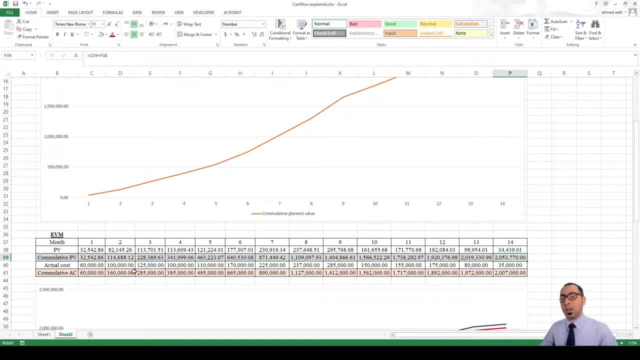 So how do we calculate the costs? Of course, Of course, and the budget will be something similar to the cost estimate or to the dry cost, but slight differences are there. So we will be discussing these in details there, But here I want to show you or make you understand the concept, guys. 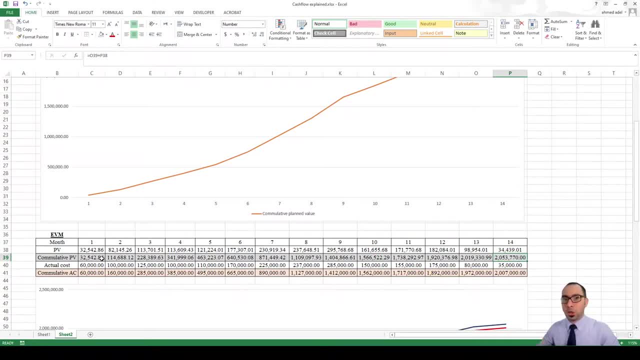 So when I, when I see how much is my budget, these are the monies that I am planning to spend on this project in order to complete it. These are my costs, not my price. OK, so I am planning to finish this project at two million and fifty three thousand, while the price of the project is two point four million. 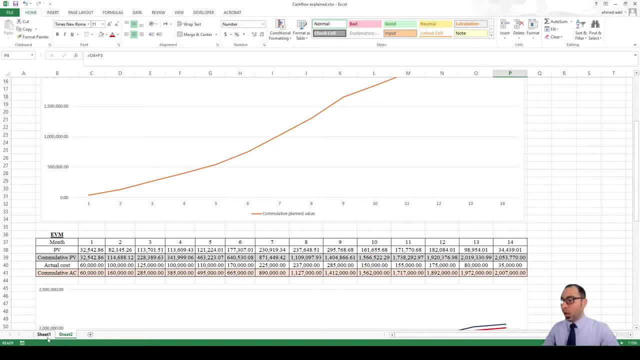 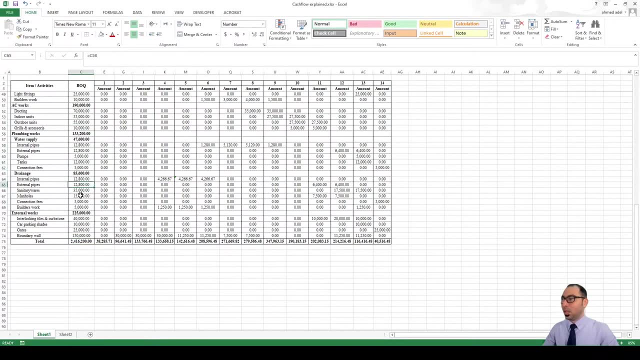 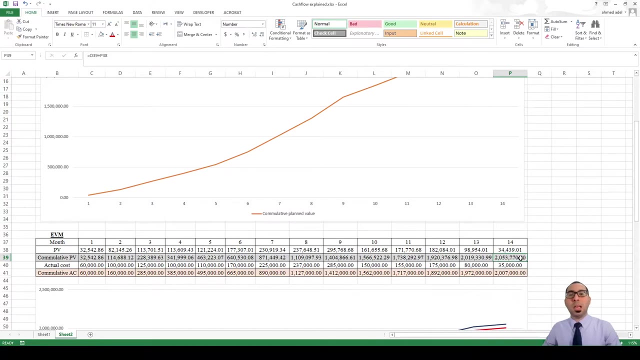 So this will be the first part, And after, when I go to this view and I start removing my margins from here, I'll get lesser than these values and the submission here will not be two point four, It will be two point zero, five, three or two million fifty three thousand. 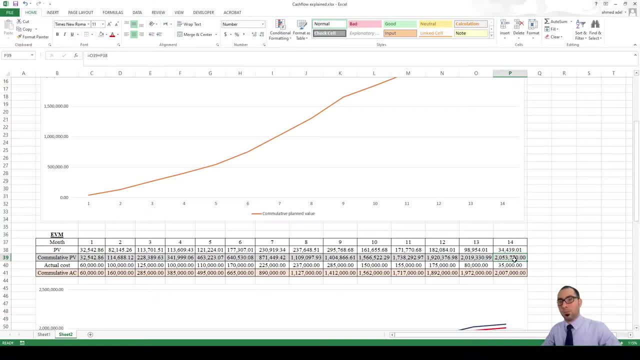 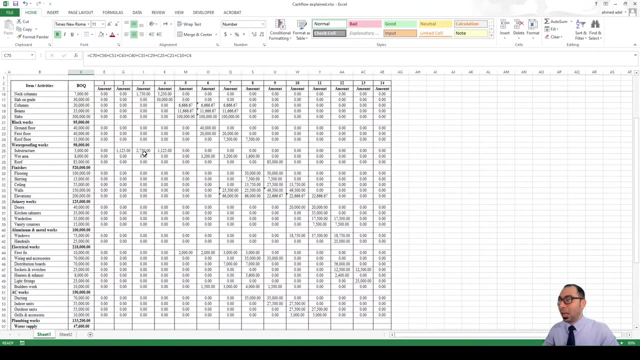 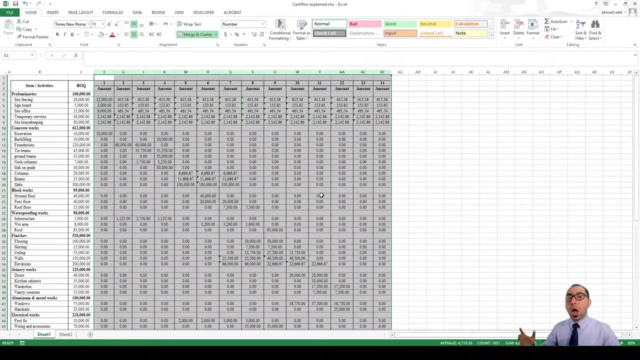 So I am planning to finish the project at two million fifty three thousand, OK, and I have a book that shows me how two point two million fifty three thousand, like I have the breakdown. So when I use the breakdown of the two million fifty three thousand and I go again and load this budget book on my schedule, OK, I'll get my internal cash flow, not the one that I give to the client here. 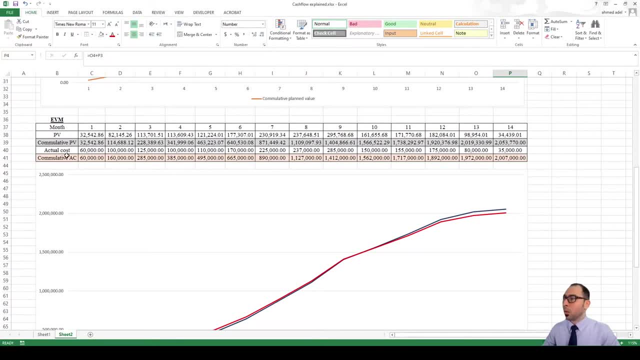 OK, I'll get my internal cash flow, not the one that I give to the client here, The one that gives two point four million. No, my plan will be to finish the project at two million fifty three thousand, And this is how. these are my planned values as per my budget. 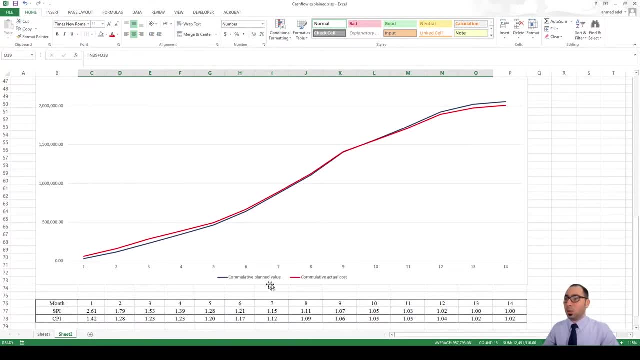 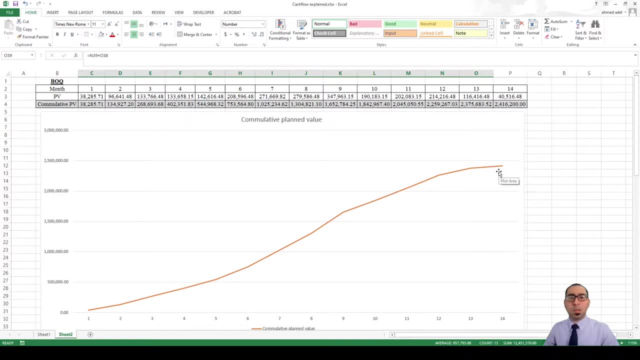 OK, and this is very important, guys, in terms- And this one is the blue line here. You see the blue line. OK, this, this blue line, is similar to this orange line, But the only difference is that here that I was doing month again. 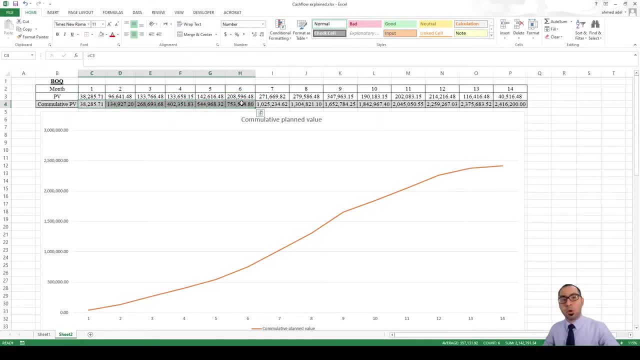 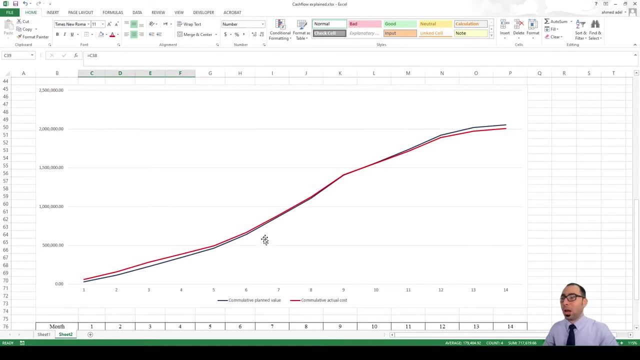 It's cumulative Planned value for the price view of you, but here I am doing month again- is the cumulative planned value of my budget view of you, and I am getting a curve that looks similar to the curve that I gave to the client and the consultant. 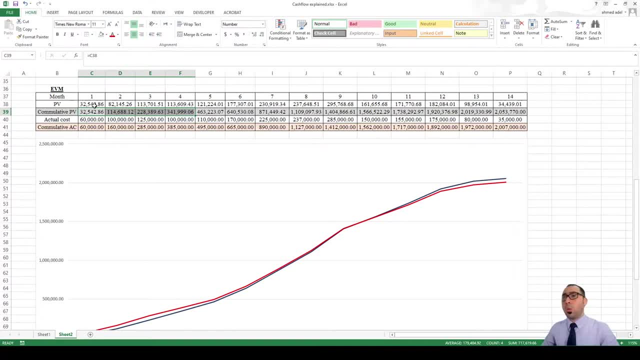 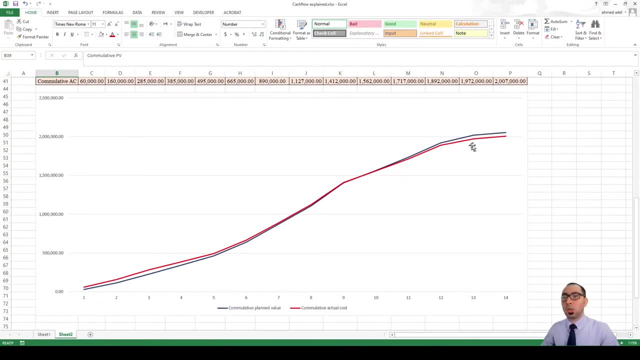 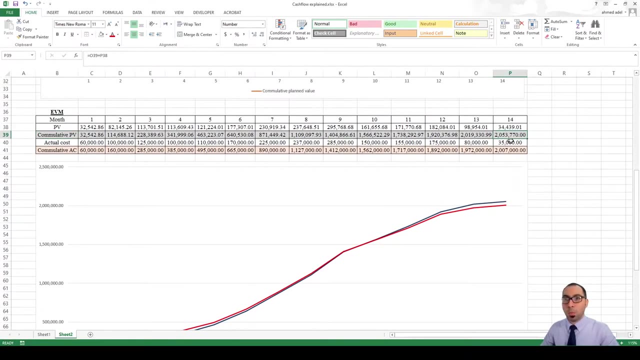 OK, So now we we finished the budget and we prepared the planned values as per the budget and we got our cost baseline as per our OK Budget. OK, And we understood what is the difference between budget or our costs, and the project price. 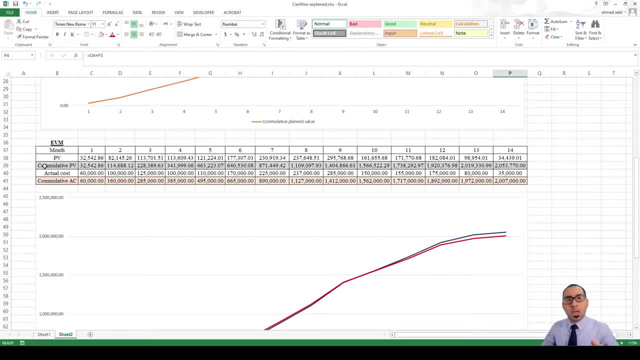 OK, guys, very good, I am seeing some of you just shaking your heads like that and not understanding our. please focus, guys. focus on what we are saying here. These are very valuable information. OK, so now we have the planned values. OK, and we have our cost baseline. 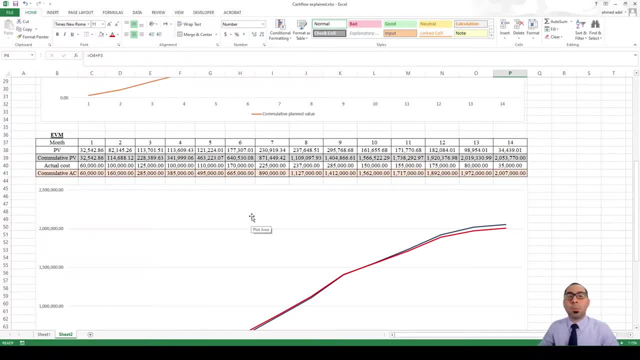 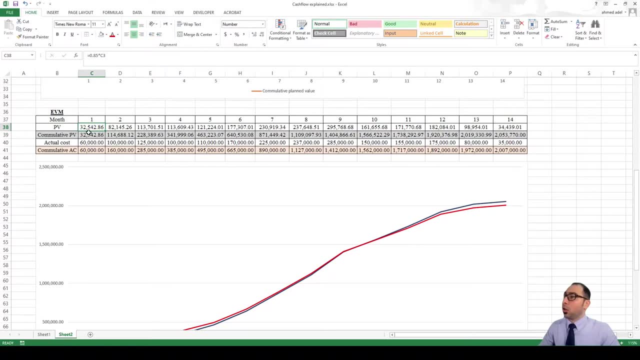 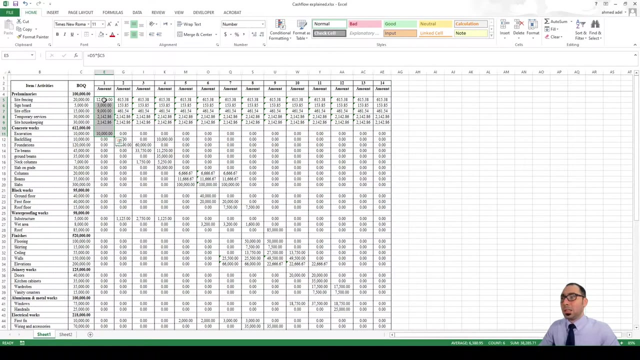 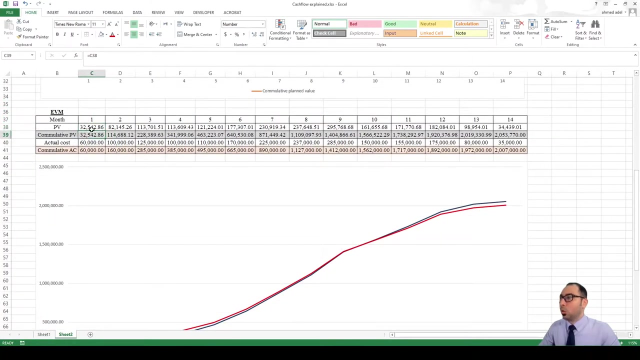 And now we will start executing the project. OK, very good. So I was planning, as per my plan OK, to execute in the first month These items. OK, which is as per my plan budget will cost thirty two thousand. 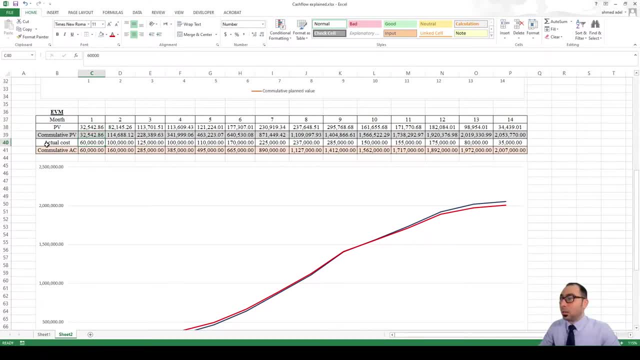 But by the end of the first month I found that The actual cost that I have encountered is sixty thousand, like I have paid sixty thousand to execute a worth of job of thirty two thousand. Oh my God, In that moment I got terminated. 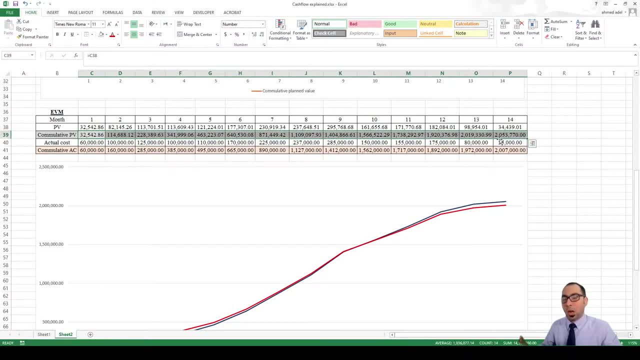 I lost my job as a project manager because the project manager will have the project budget and he will execute accordingly. So if I am the project manager- and this is my case- my planned value for the first month Is thirty two And I ended up spending sixty thousand. 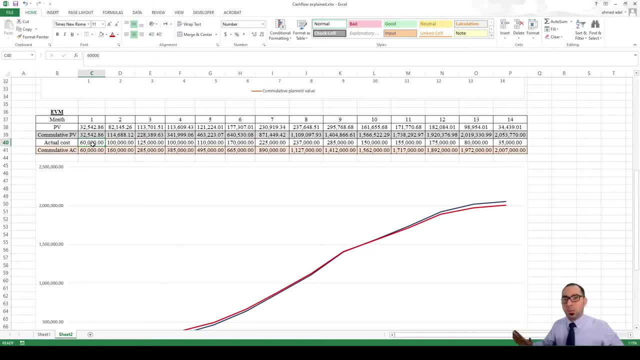 Oh my God, I am terminated. I lost my job, Is it true? Because here and I will keep updating the costs every month. So if I every month again, this is the planned value, that the worth of what I will do every month. 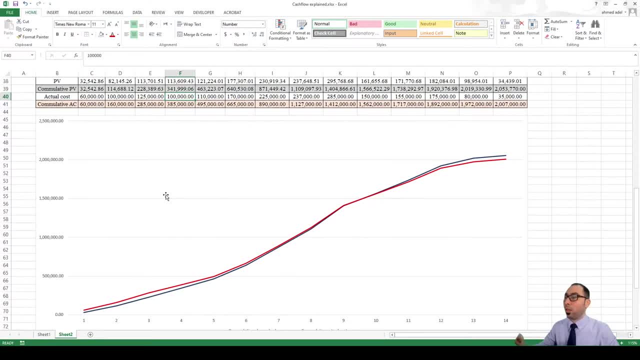 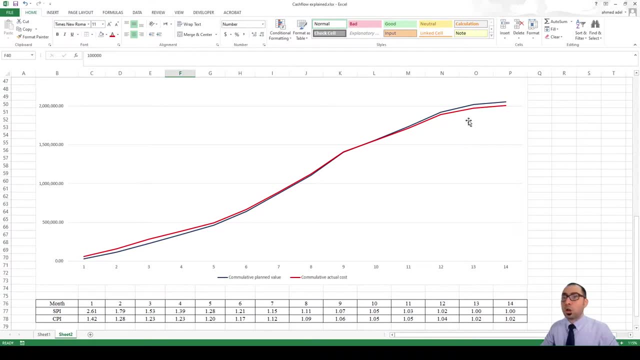 And again is that I am putting my actual cost every month. So you can see the blue line is the cumulative planned value. So if I, but the red line is the cumulative actual cost, okay, so you can see here that by the end of the 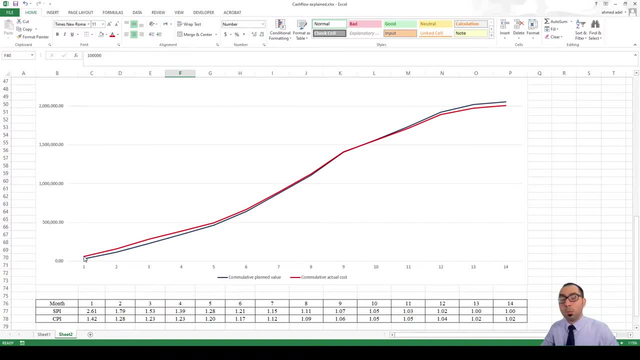 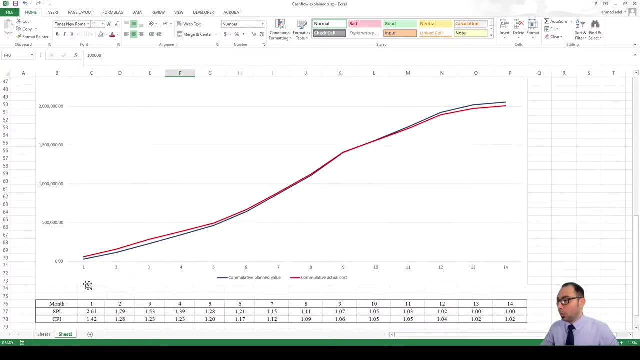 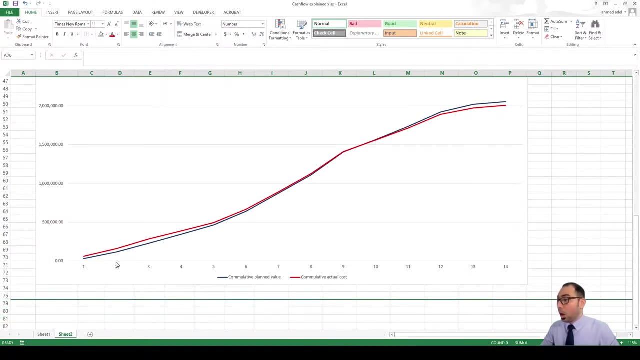 first month i should spend up to here, but i spend it more, oh my god. second month: same. i should spend this much only. but okay, let's hide this, because hide again by the end of the second month, what i was supposed to spend this much. i'm spending more. third month more, fourth, more- oh my god i. 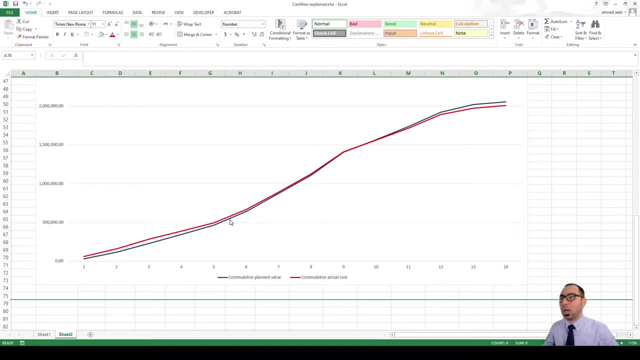 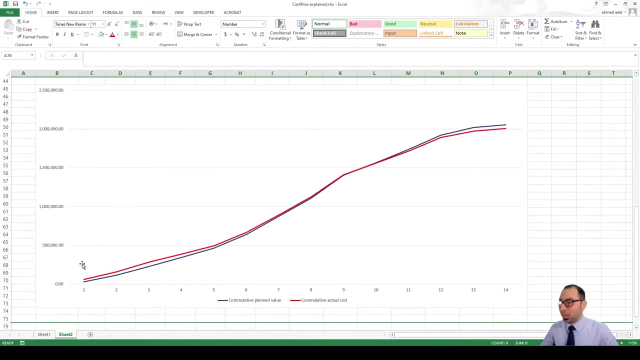 am losing. now i am losing why i am over budget, guys. my actual cost is more than my planned value, okay, so now the question to you guys is- and i want you to pause the video and ask yourself this question now: as per this that you are seeing here, did i win or lose in the end? 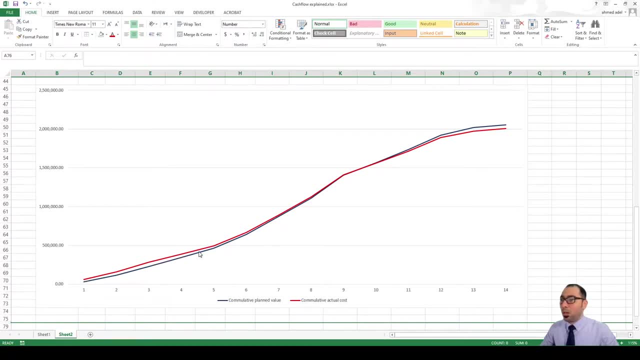 if i tell you guys that all this period, i am spending more than what i have planned to spend and only starting from here i started to spend less than what i have planned. okay, so some of you might think that we are losing. in that case, why? because you see, this area, the 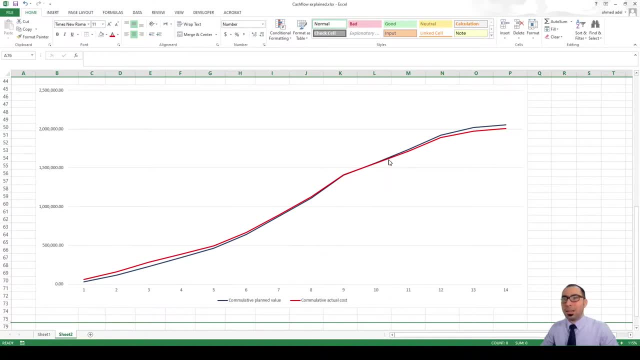 area between the lines here is bigger than the area between the lines here seems like i have lost it. so for me, i have invested and i'm set in the middle of the can, so the balance is the same. i live more then and i arm again on the upper side. 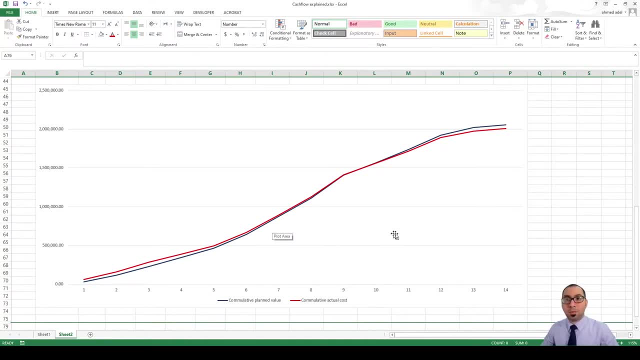 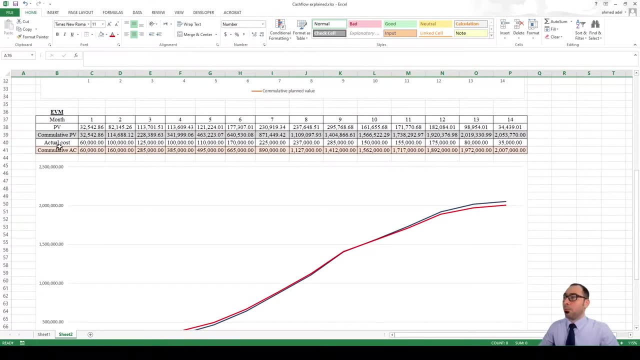 over the part here, and that means that i have spent here more, and this is this part that i have saved is less, so it didn't cover this part and it means that i have lost. well, this is not the case. guys actually value management. now you have planned to spend 32,000 by the end of the first. 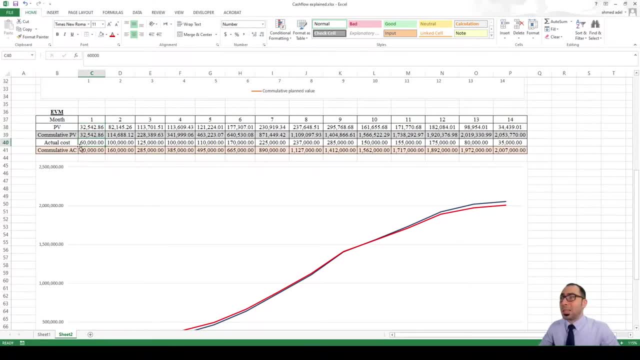 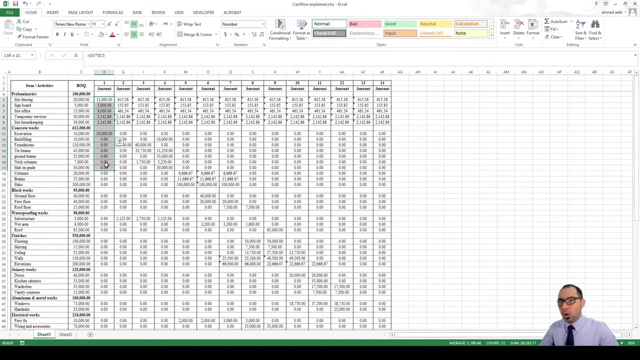 month, but you ended up spending 60,000 by the end of the first month. but you need to ask yourself a question: why did I spend 60,000 out of my POQ budget? POQ- what are the items that I have really completed? did I complete only? 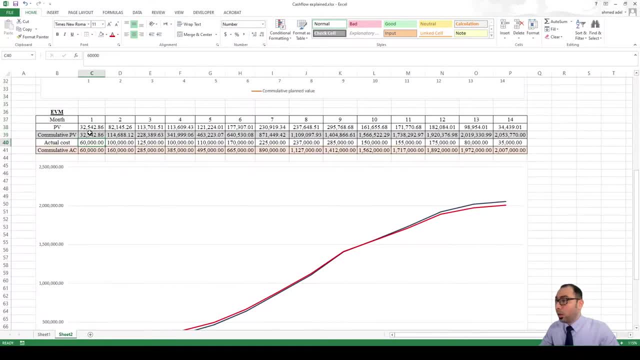 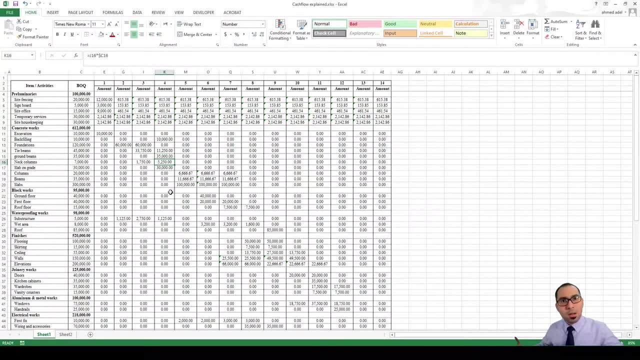 these five or six items that is worth 32,000, or did I complete something more? did I go ahead of my program, and that's why I am spending more. what did I earn, guys? why I am spending more. this is where you go to the here. let's unhide. 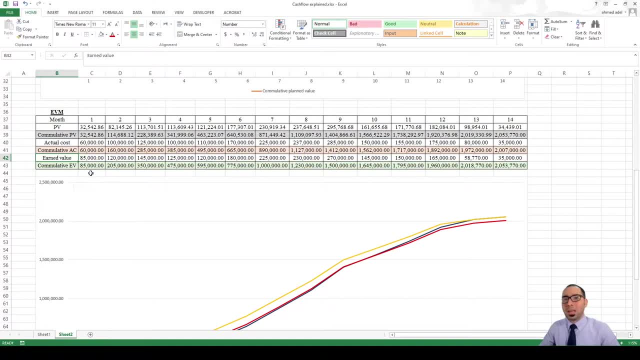 it, the earned value. what is the earned value, guys? this is the value of works that you have completed by the end of the first month. so your plan, your plan from your budget POQ, which is here- your plan was to finish 32,000 worth of. 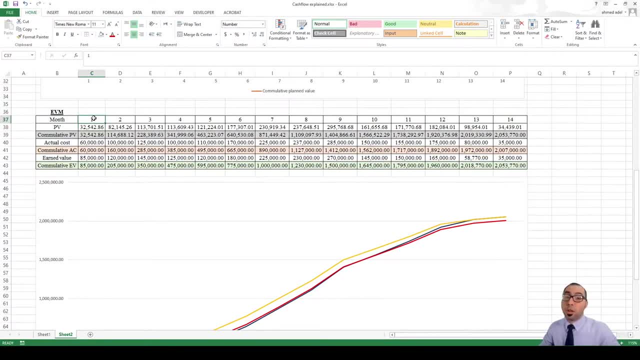 works by the end of the first month. good, this was your plan, but what happened? you found that you have spent 60,000. okay, and you will get worried. oh my god, my cost is more than my planned value. so what, you might have executed some items. 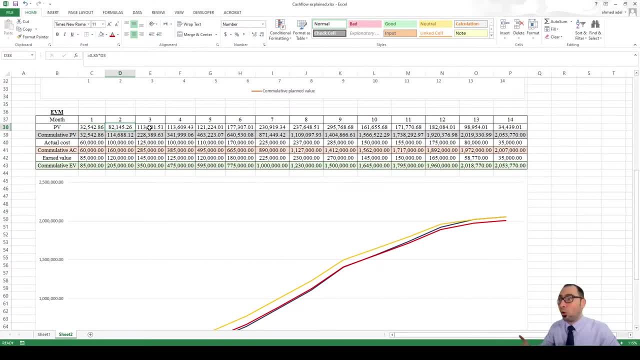 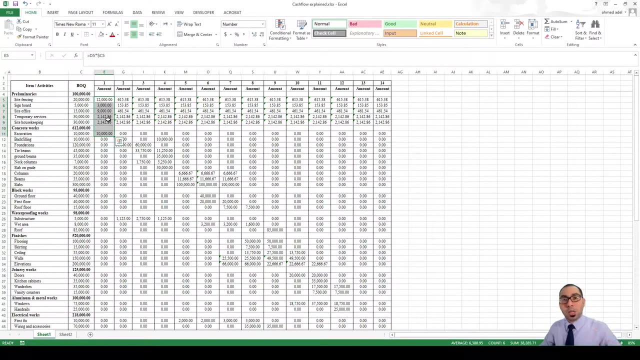 that you have planned to execute in the month number two or month number three. you have executed them here. so you need to go back and you need to see how much is your earned value like out of your POQ items. did you really execute these items that you have planned to execute in the first month only, or did you? 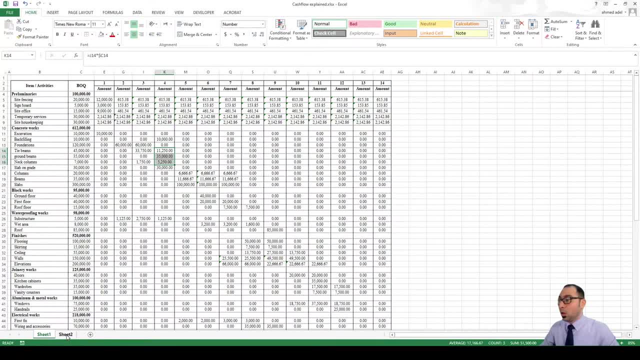 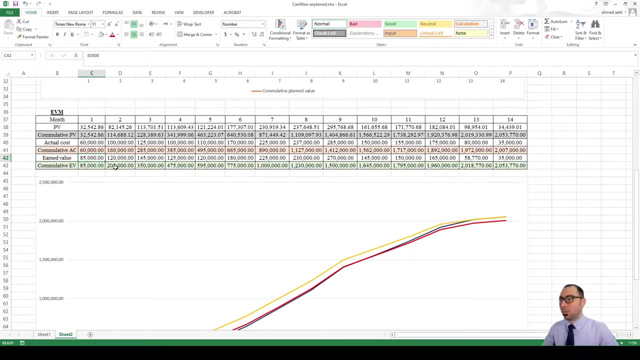 execute something else from these activities. so here I can see that I didn't finish only these five or six items that are planned to be 32,000. no, I finished more. I finished 85,000 worth of works. so what is happening here? this is: 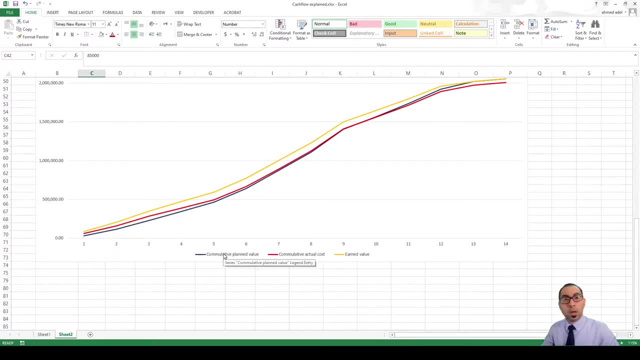 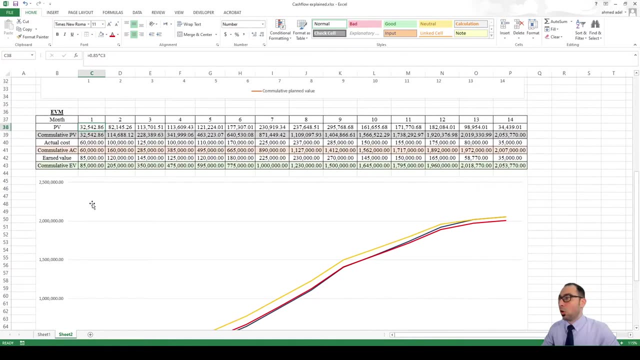 my planned value. my planned value is that blue line, so I was supposed to spend 32 but I ended up spending 60. so if I don't know how much is my earned value, what is the percentage of works that I have completed? is it more than the 60 or less? I will not be able to make a judgment if 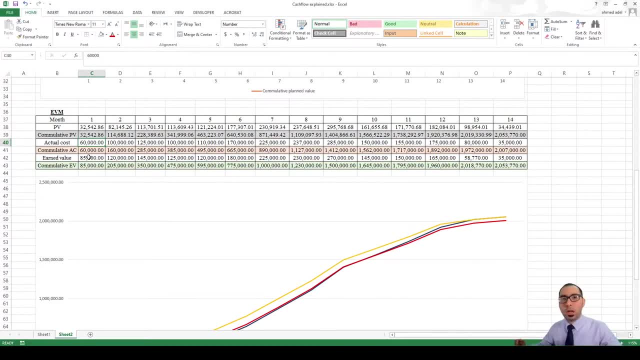 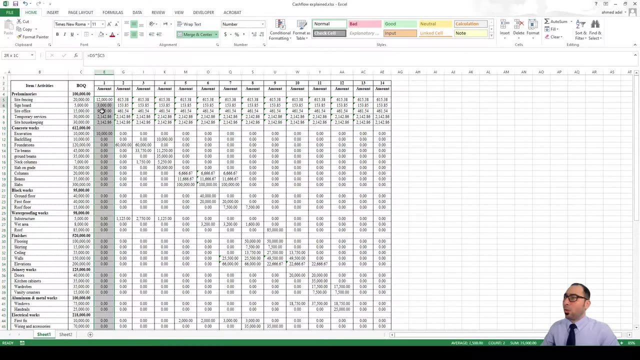 I, if I am doing my project on the right way or not. okay. so this is what we call guys: the earned value. the earned value simply is the percentage of works completed, and what does that mean? my plan was to finish these items in the first month, but I have finished more. I did, I did more. 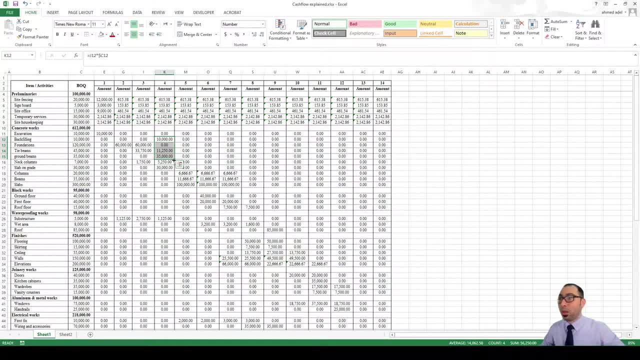 things that I have planned to execute in the second month and in the third month and in the fourth month. maybe I have executed a part of these works or all of them here, so that means that I am ahead of my schedule. I am like I I did. 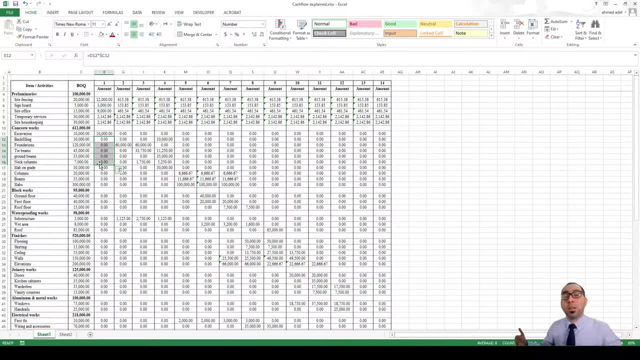 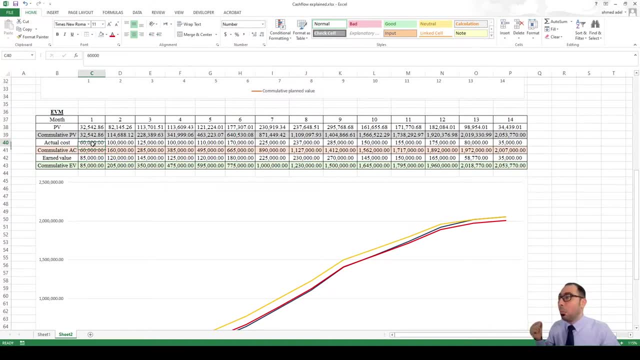 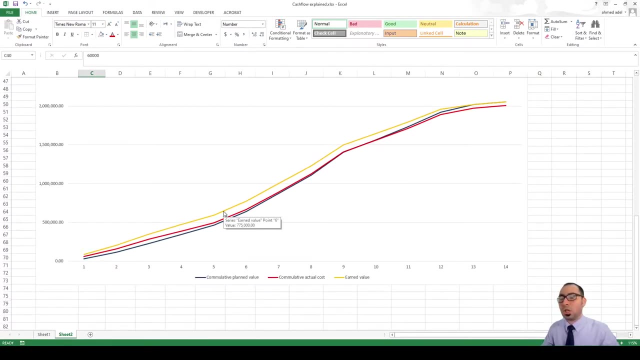 something now that I should have done next month or after two months or after three months, and that's why I am spending more, but actually I am earning more than I am spending. so I am in a very good position. so when I have this third line here, which is the earned value, I can say that 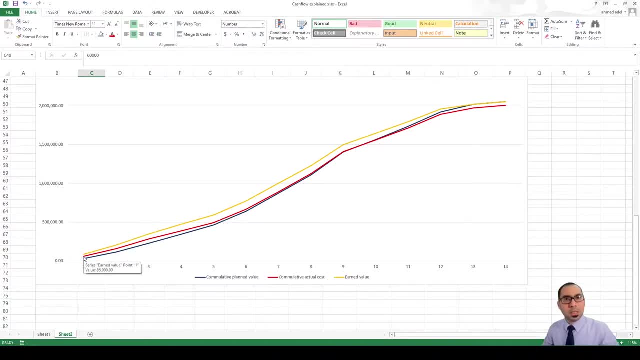 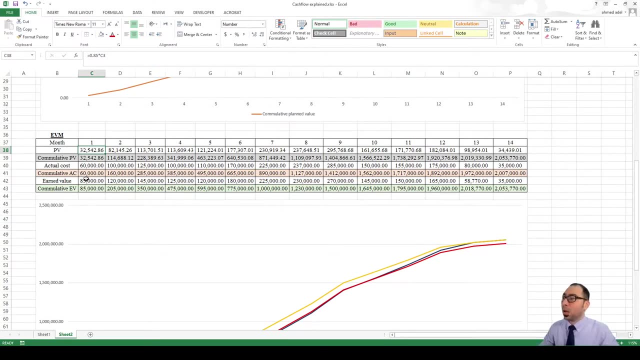 the planned value was this: I spent 60,000, yes, but I earned 85 instead of earning only 32. that I have planned, guys. so here, second month again, I was supposed to finish 82,000 worth of job, but I've ended up spending 100,000. 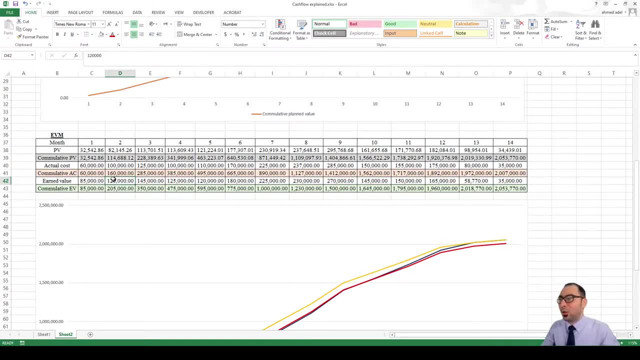 am I losing? no, look at your earned value. you did a worth of words, 120,000 worth of words. so still, you, you are earning more than you are spending. so that means that you have cost under run. okay, you are like you were supposed to like your, your plan. 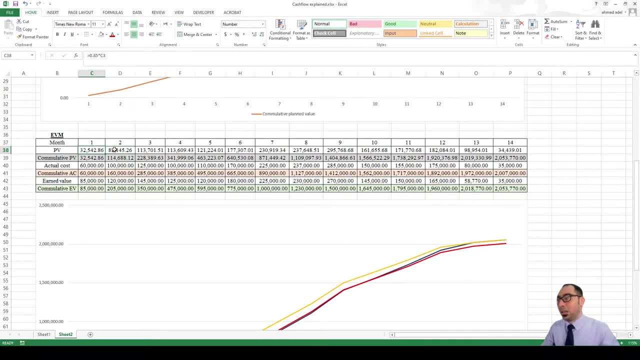 was to do these works okay at these costs. you encountered more costs, but you didn't achieve these two numbers. you achieved more, so that's good. your earned value, or the percentage of work completed, is much more than the plan and you are earning more than you are spending. you are actually winning. but if 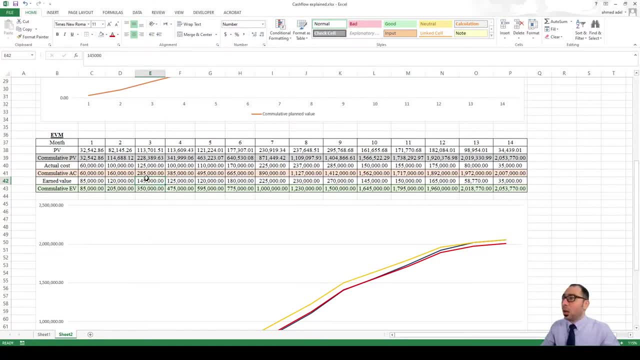 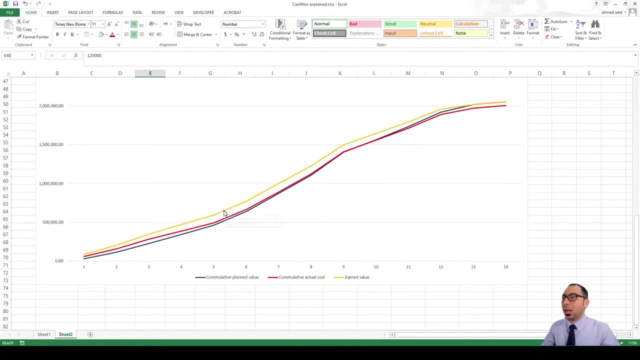 you keep doing that every month. okay, the earned value is more than the actual cost, so this yellow curve will start going, going and it is. you see, it is up always. it is above the other two curves. okay, above, above, above. you cannot continue like that forever, guys, because in the end, in the end, you 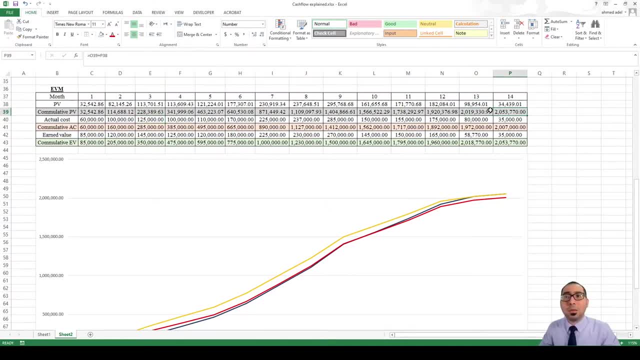 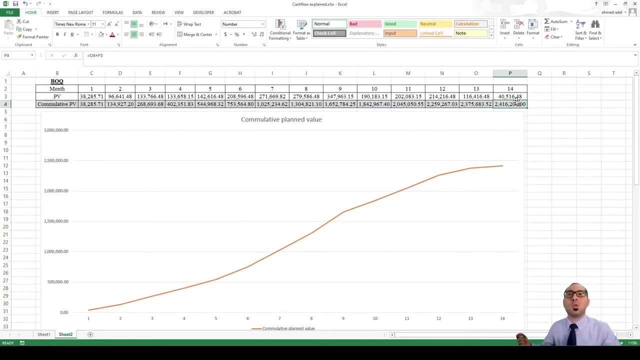 have budgeted your project at 2 million fifty three thousand. so by the end of the project your earned value will be a hundred percent of this number and in the end you you have done your budget. you know that your project price is 2.4 million. 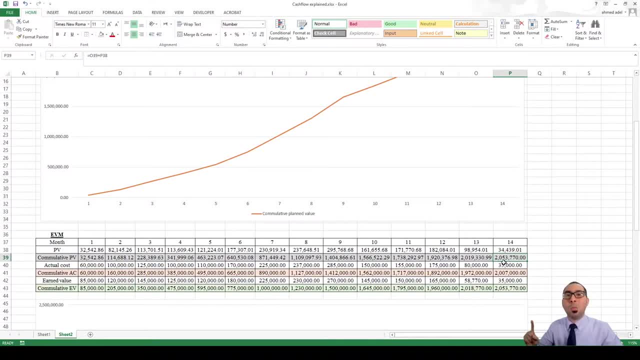 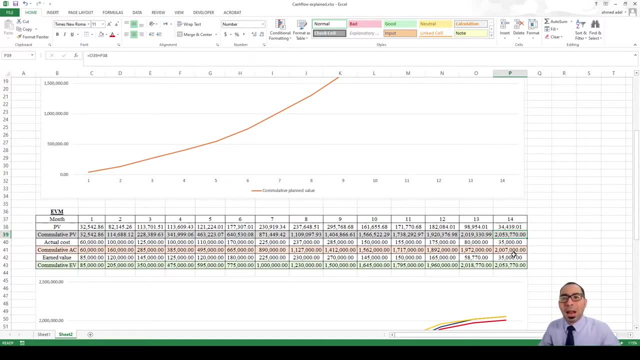 but you said i will finish this project at 2 million 53 000. good, okay, so when you finish the project, it doesn't matter how much you your actual cost is. you have earned the number that you have set for yourself. so that means that you have completed 100 percent of your planned value. 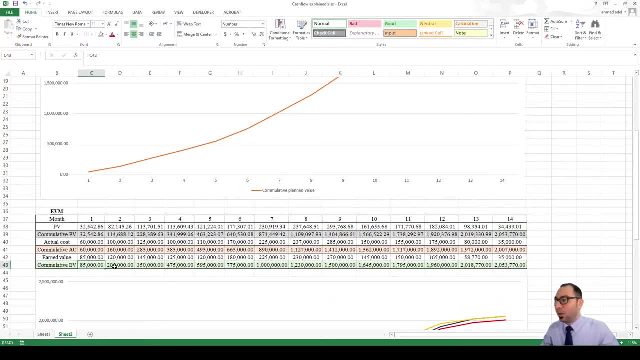 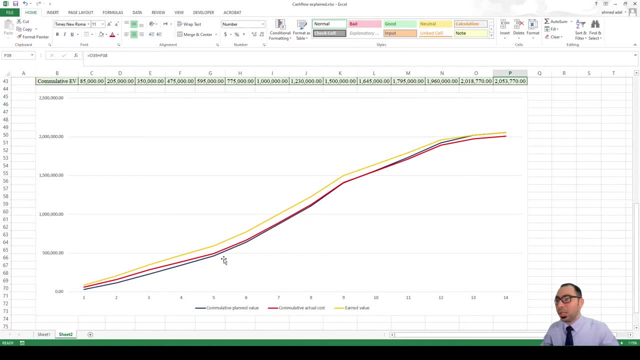 okay. so that's why here the cumulative earned value, okay, will reach to the same planned value in the end. the blue line, which is the planned value and the earned value, will, like, definitely intersect here in the end. okay, but what about our cost, guys? our cost was higher than our planned. 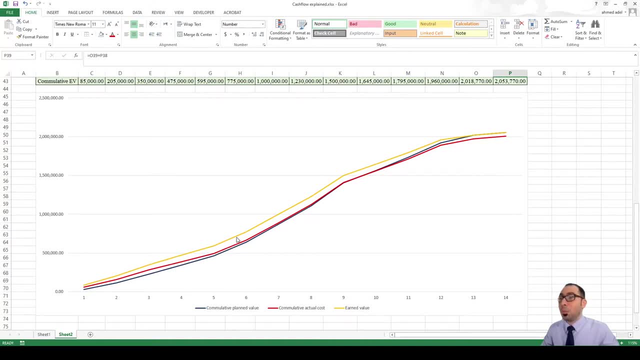 value here all the way, but we were earning more than what we were spending on the project. so that's why we have the cumulative earned value okay, so that's why we are spending okay, but in the end our planned value here is our budget. it means we met our 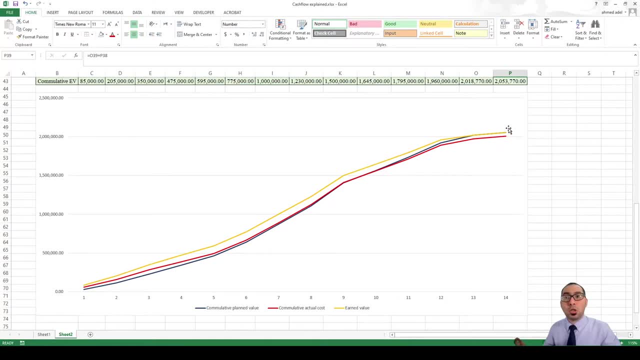 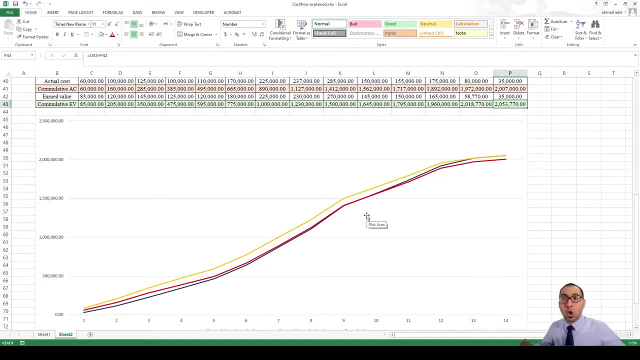 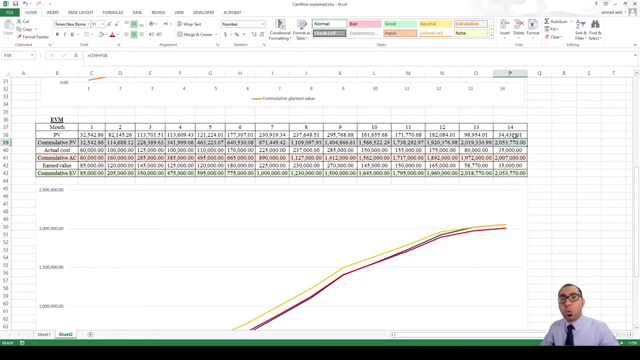 budget okay, but our plan to reach this number, which is 2 million 53, was changed during execution because we were ahead of our schedule. plus plus. i was budgeting for myself that i am going to finish the works at 2 million 53 000 and it didn't happen. i finished the works at 2 million only. 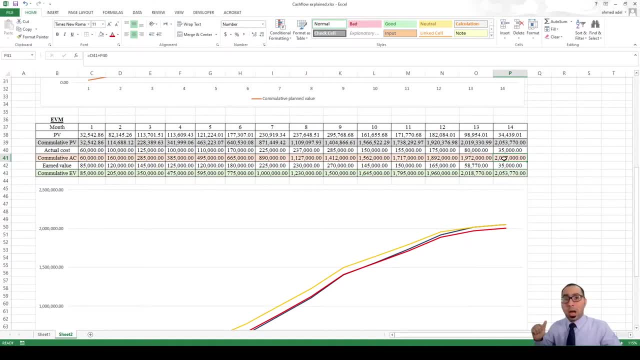 guys. so i have like cost on the run. i i didn't exceed my budget. this is number one and number two: i um finished at uh on time, like in the in the 14th month i finished all the the works, so that means that i met my schedule as well and, as you know, guys, the earned value and the actual cost. 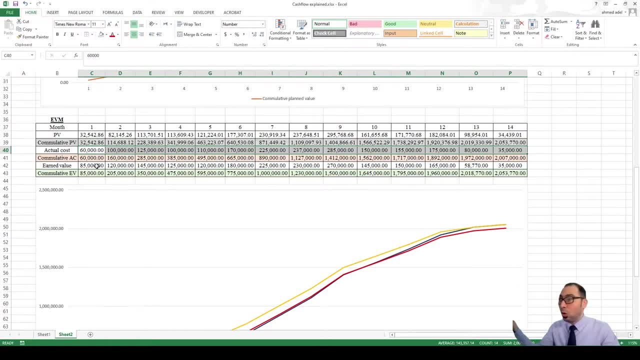 it will not. these details will not be available to you from the first day in the project. no tá, the only thing that you will have in the first day in the project is your planned value. these, this is your plan. this, these are the monthly numbers and this is that cumulative. this, what? 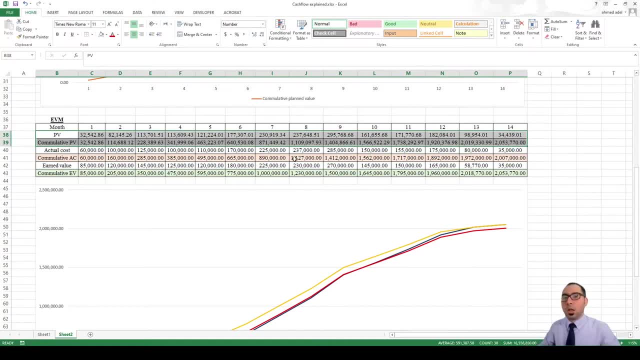 you will have in day one. but by the end of the first month you will go and calculate your costs. so my my actual cost or i spend in. in the first month i spend 60 000 and you will calculate the percentage completed of your budget and you will see that you have completed works that worth 85 000. 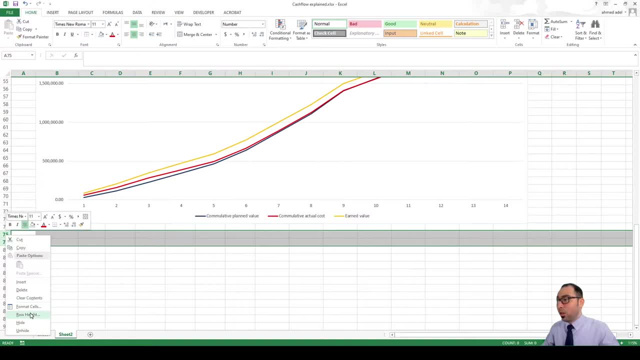 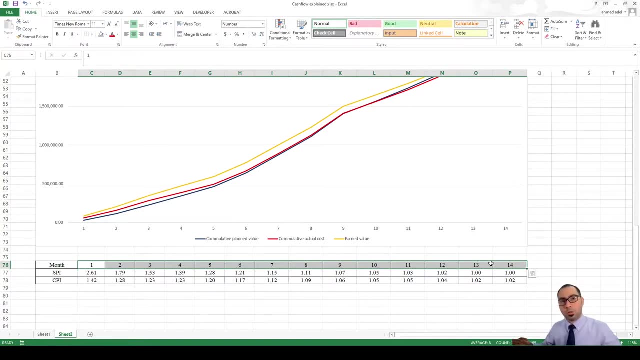 so you can, in the by the end of the first month you will be doing this. and here again, these are the months. okay, 14 month, which is our duration to execute the works, and we have two things that we will keep monitoring, like all along, as long as we execute every month. we will be monitoring these. 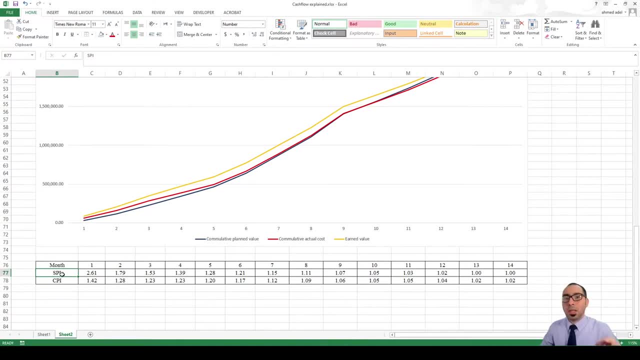 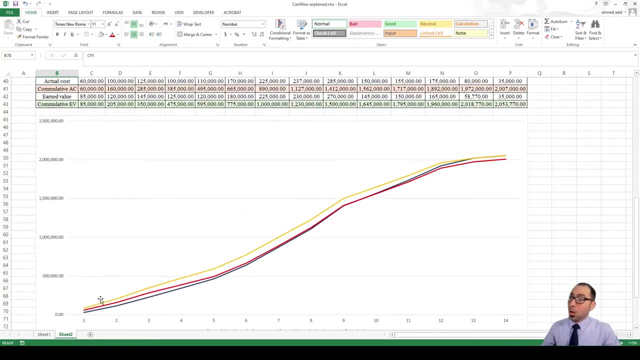 two periods of each month and our total minimum is 99: 00. coherence with the presentation, things, things. and what are these two things? something called schedule performance index and the other one is called cost performance index. so here guys, what, what are these two things mean? actually, we 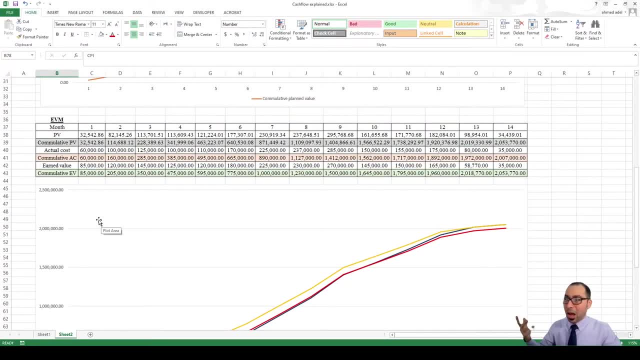 have discussed this, but i will, like you, have an idea now. my planned value, or i was planning to finish 32 000 worth of works by the end of the first month, but i finished. i finished 85 000 worth of words. let me close this because we don't need any disturbance. okay, back to what we were saying. 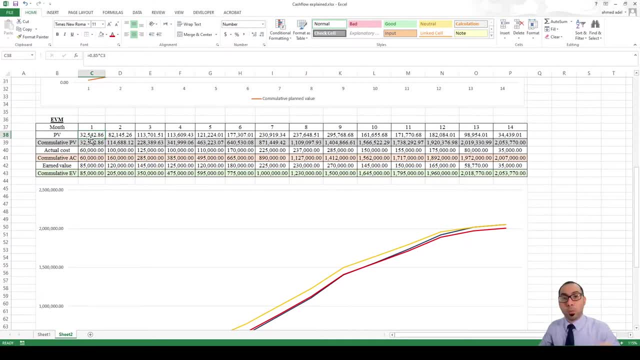 the planned value here was 32 000. you were planning to finish 32 000 worth of works, uh, by the end of the first month. but what? what you have done? you have finished 85 000 worth of of works, as per your budget, or your budget BOQ, and you spent 60,000.. So you will calculate these. 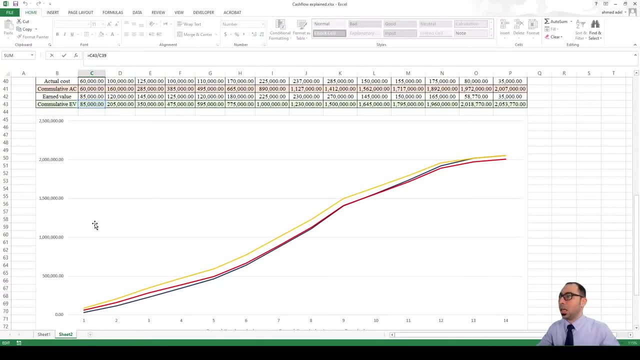 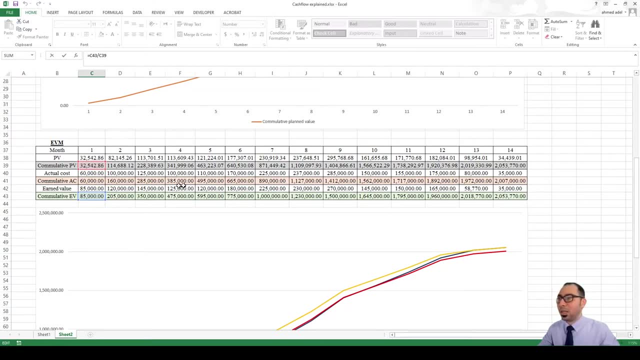 two index here. Scheduled performance index, guys, is equal to the earned value divided by the planned value in the first month. because you don't have these numbers yet, We are now making the evaluation by the end of the first month. So cumulative value, or cumulative earned value divided by the 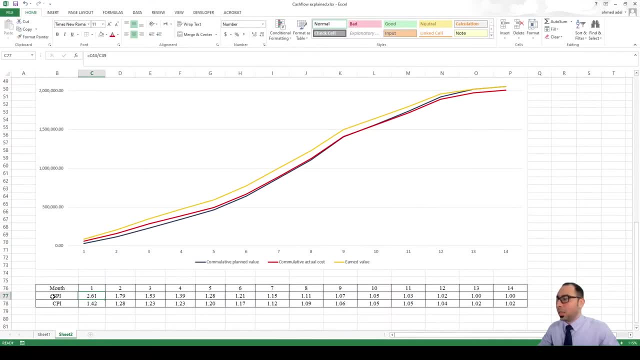 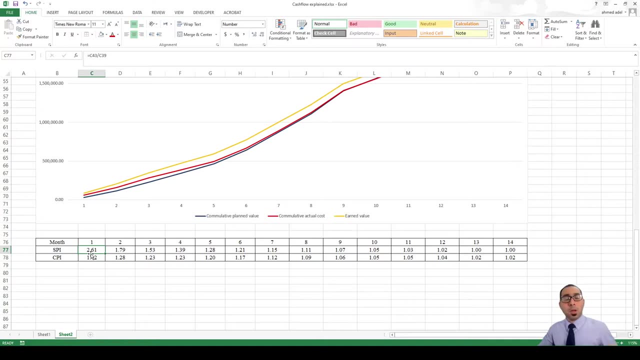 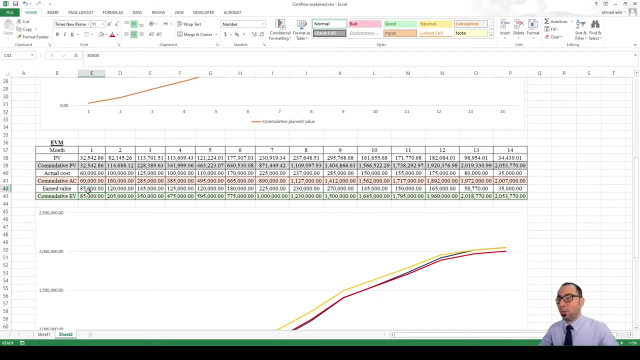 cumulative planned value. I am getting here a scheduled performance index of 2.6, which means I am 2.6 times ahead of my schedule. I am ahead of the schedule I was supposed like if you finish here, if your earned value by the end of the first month is 32 only instead of 85 and your planned 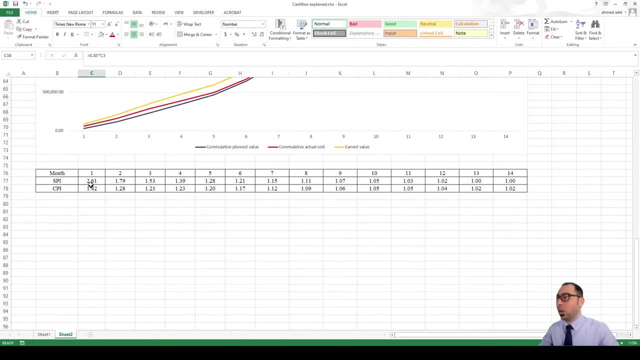 value is also 32. So when you divide this by this, you get here one. One means that you are on time, that you are following your project, You don't have any delays and you are not ahead of your schedule. You are on your schedule. But when this number is more than 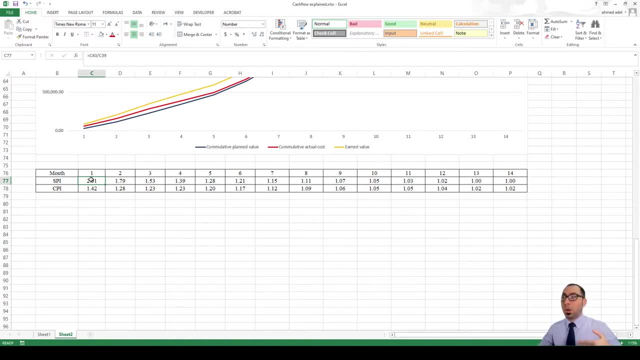 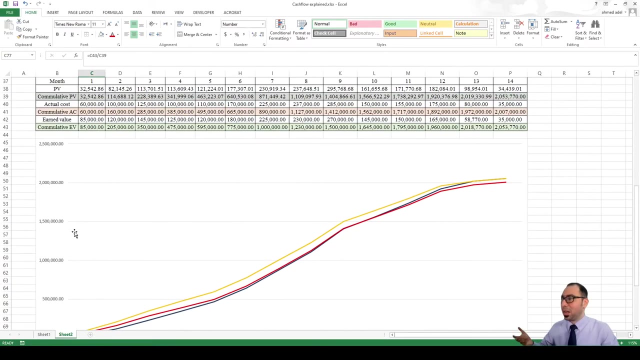 one. it means that you are ahead of a schedule, But ahead of a schedule by how much? By two and a half times more. This is 261 percent ahead of a schedule, guys, which is amazing, okay, For example, in that case, maybe in in your, in your real life scenario, the variance will not be that much like. 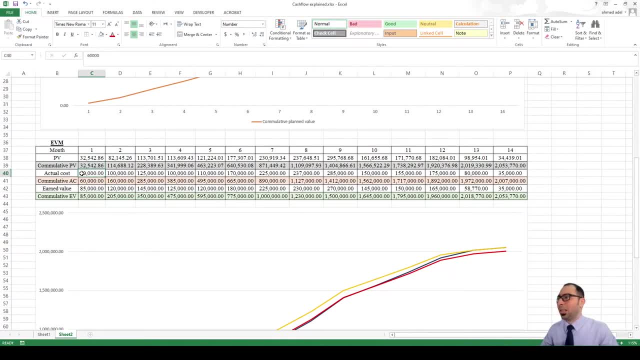 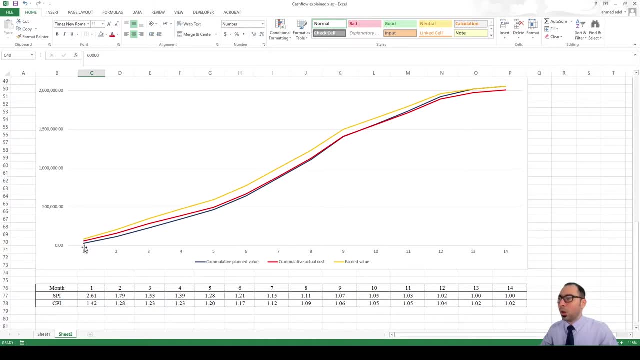 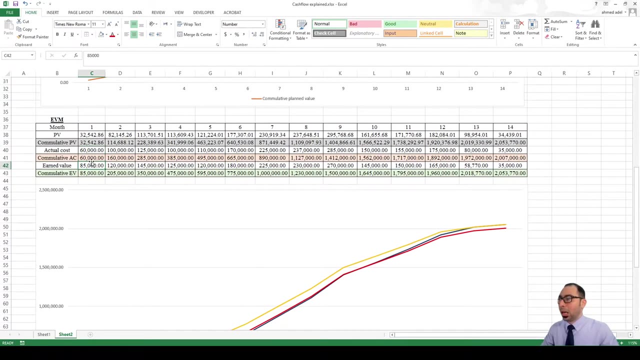 you plan 32, maybe you will spend, let's say, 32, and you will earn maybe 35. But if I did my example like that, these three points will be like very near to each other. I won't be able to explain the difference to you guys. That's why I kept like a big difference here between the three values. so 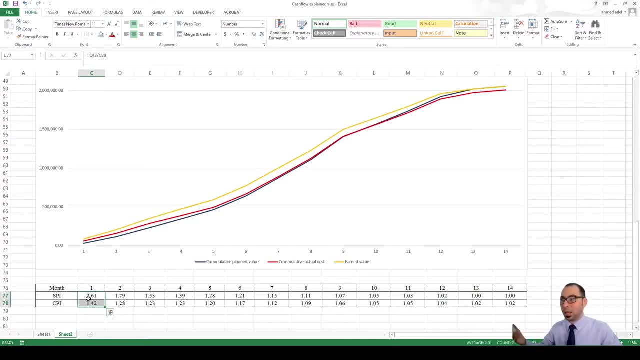 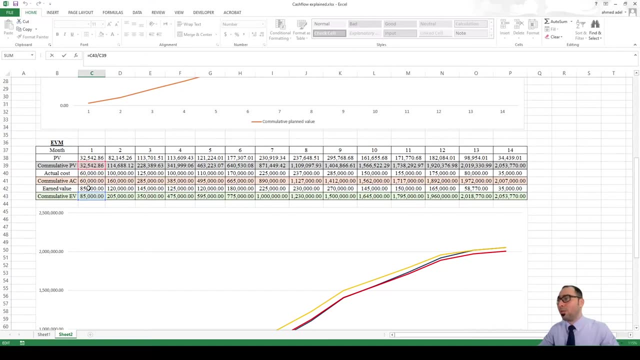 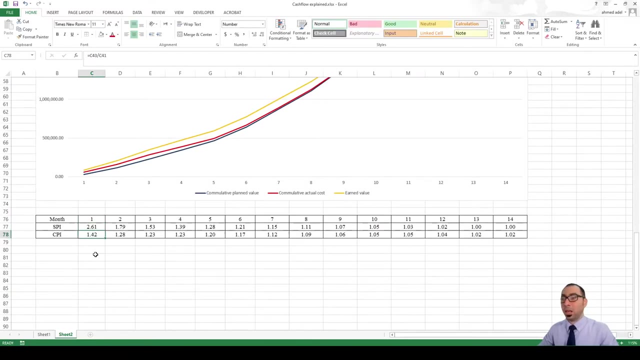 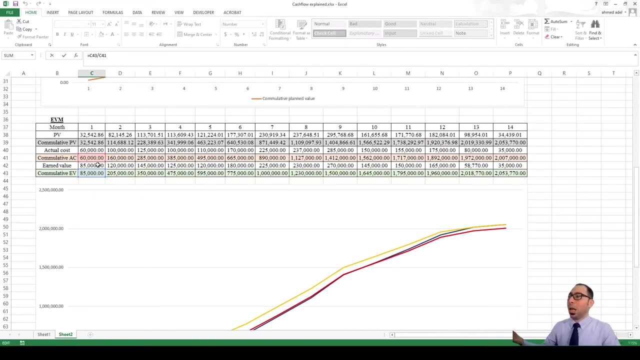 that this can be clear and to also explain the end. So again, schedule performance index is earned value divided by planned value, Cumulative, or, like the, the monthly one. Okay, what about cost performance index? Cost performance index is the earned value divided by the actual cost. Because what happened? the cost, the cost of the works that 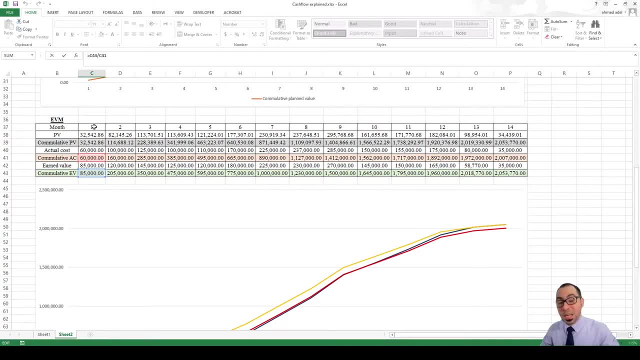 I have finished in the. in the first month, the cost of these works should be 85. 000 guys, Because my BOQ, my budget BOQ, says that if you finish these 10 items, you get 85 000 as per your budget. But what happened? I finished these items, that gives me 85 000, but I spent only 60 000. 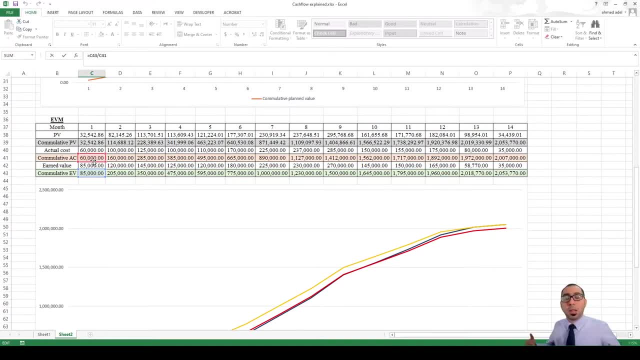 So that means I'm having cost under run. I am under budget, I am under my budget. My budget for the works that I have finished in the first month is 85. But I didn't pay 85. I paid only 60.. 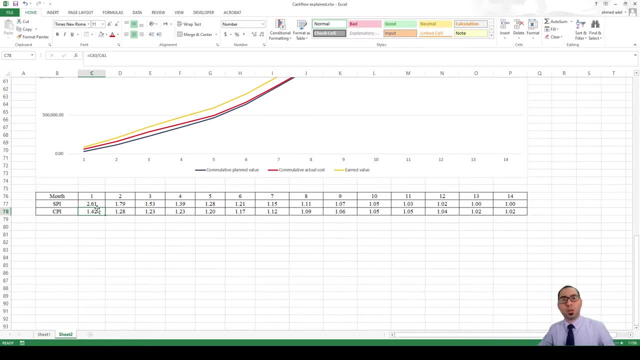 So again, the cost performance index is 1.4. That means that I have cost under run, I am under my cost, I am very like effective, or or my works are going in a very good way. And why I am telling you this? because by the end of the first month you will not have these figures, guys. So you can do. 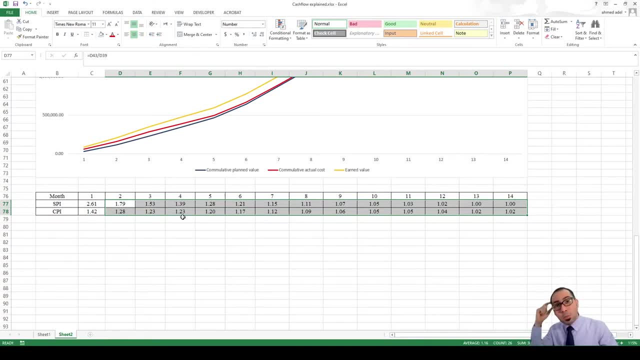 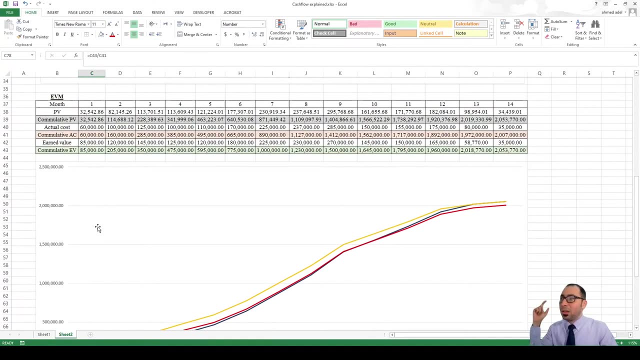 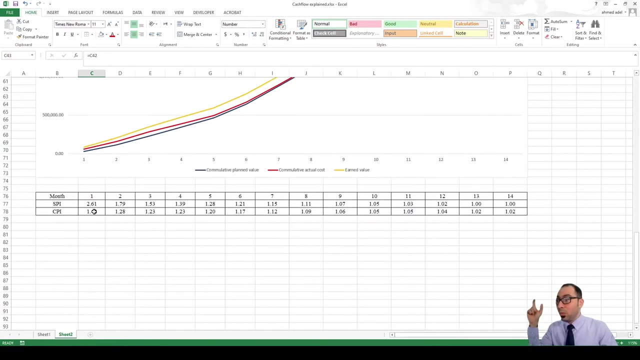 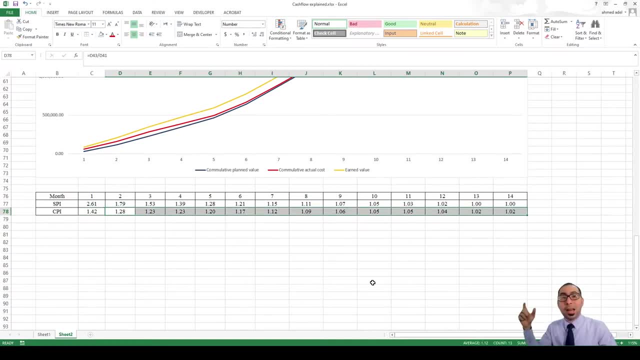 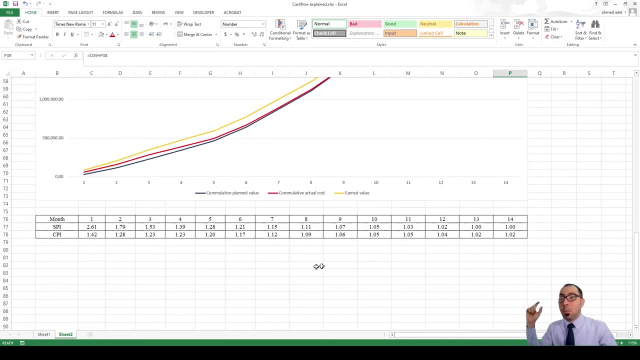 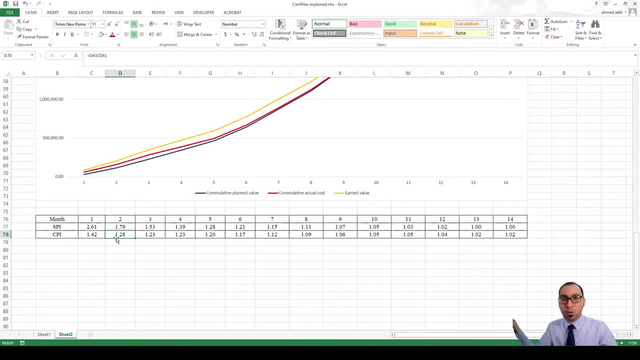 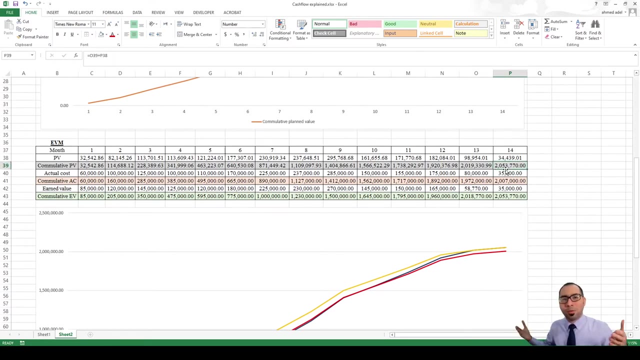 cost under run. It is not overrun, So you are not above your budget, You are below your budget. You are good, But the cost performance index is like decreasing, decreasing, decreasing, guys, Okay, Because again there is a limit, Because you budgeted to, to, to, like you did some kind of 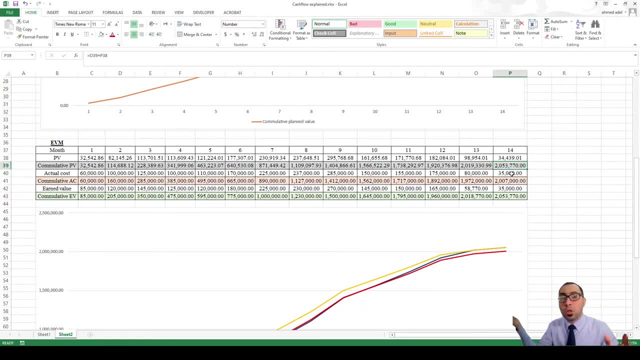 estimation or budget to understand that you are going to execute these works at 2 million 3.. So you will not execute these works at 1 million guys. It means that your estimation was wrong in the beginning. You might save something. Maybe this 50,000 you will save. You will save, maybe 20,000 you will. 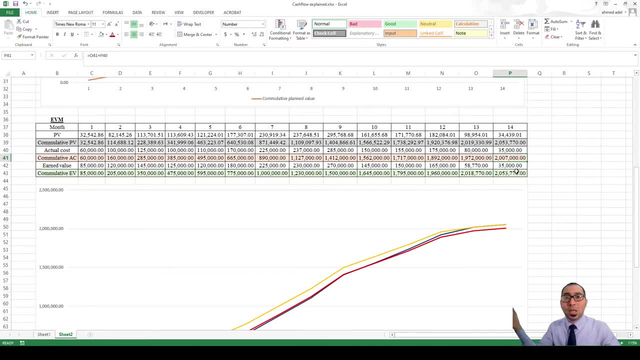 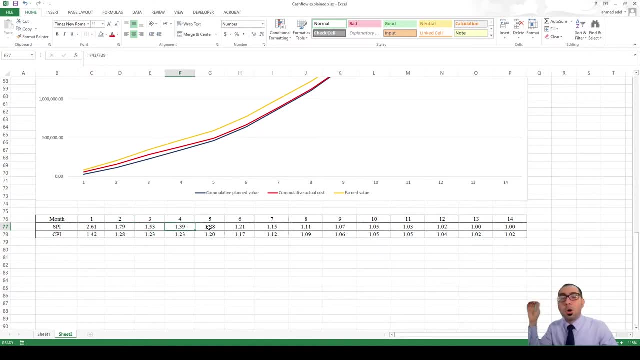 save in the end, But you will not know how much exactly did you spend until you reach here. But all the way until you reach there, you will be monitoring yourself. Am I ahead of the schedule? If this figure is more than one, it means that yes. 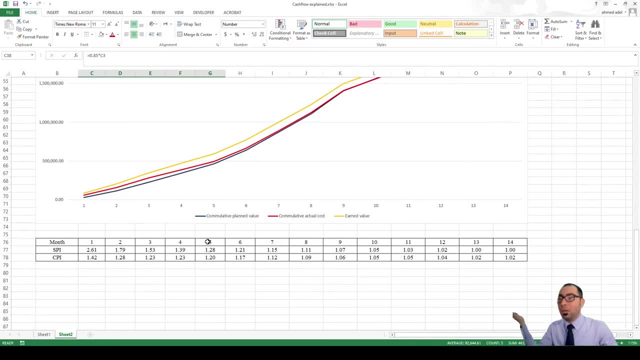 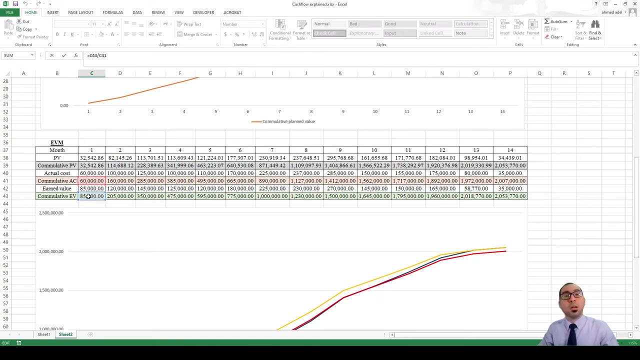 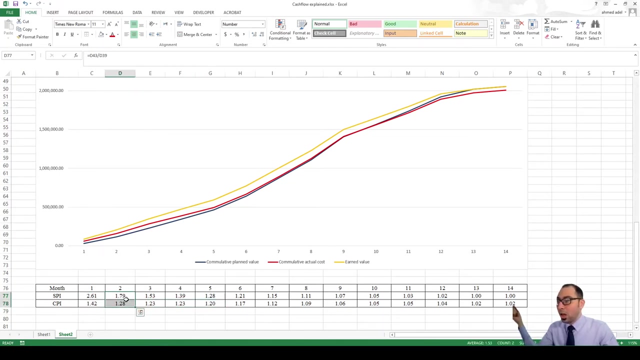 You are ahead of your planned values. And am I having cost under run? Am I under my budget? Yes, Because, again, the cost performance index, which is the earned value divided by the actual cost, I am earning more than I am spending to earn this, So it is more than one, So that means that I am good. So when you do this calculation every month, you are 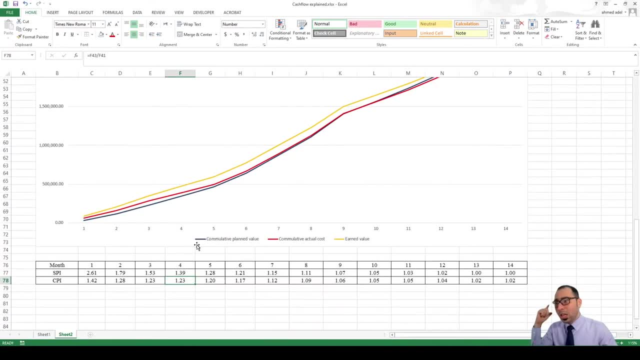 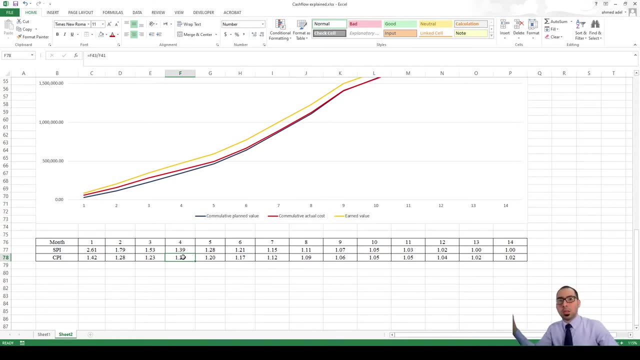 controlling the costs. So what if you came in one month and you have a budget of 1 million And you found that your cost performance index is below one less than one? That means that you are spending more than you are earning, And in that case you have to look at the side. what is happening? Why are we losing? We have budgeted these works to be. 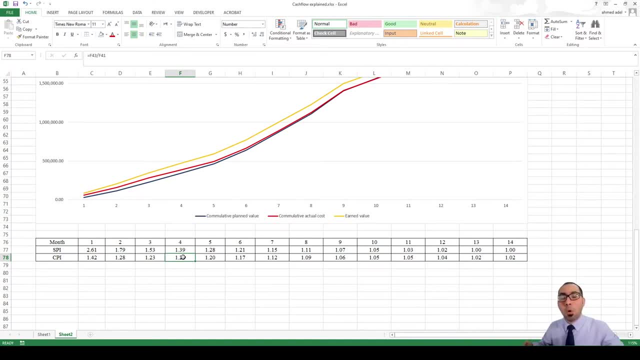 executed at this cost. Why are we spending more to execute these items? And from that you investigate the problem. You will try to solve the problem in order to make sure that the cost performance index is below one problem, in order to make sure that the cost performance index goes up above one again. and 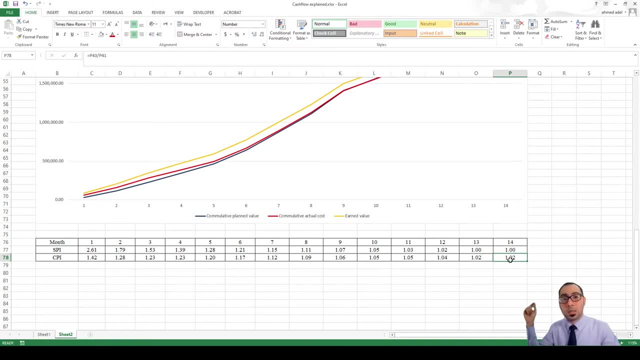 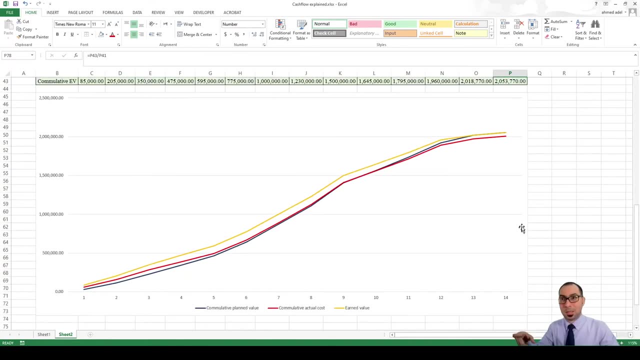 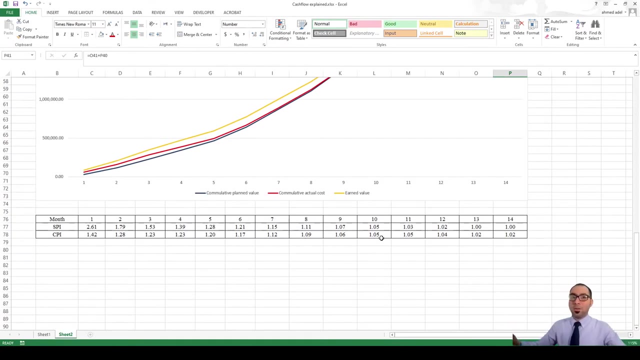 that you will finish your project at least at the budget that you have set for yourself to finish the works at from the beginning, if not less, as this case, that we have achieved a saving here, guys, i hope that the earned value management is is very clear now and you understand it very well. 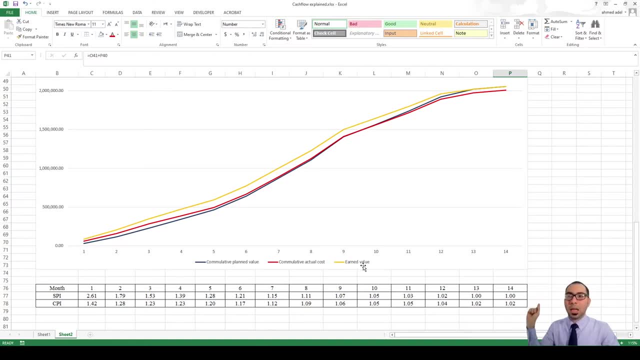 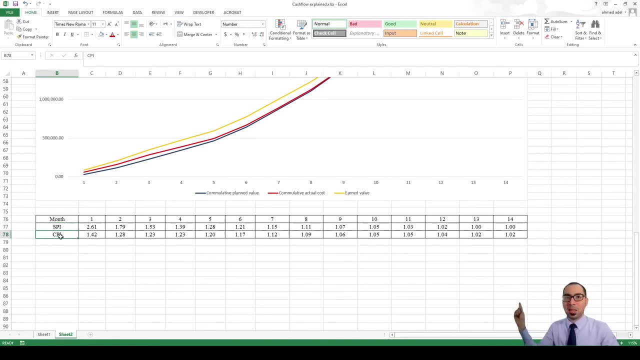 what is the planned value, what is the actual cost and what is the earned value and what are the schedule performance index? what is the cost performance index? what is the estimate to complete? actually, we have not discussed that in detail. this will be discussed in in more deeper. 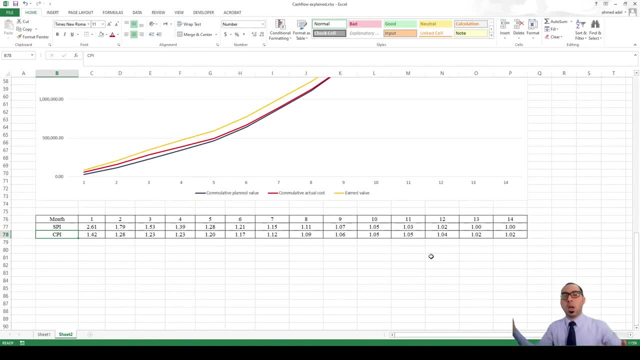 detail how these, all these numbers came from and everything in our course. number four, which is cost estimation, guys, and in the end i am very happy and i hope you didn't have headache from my shouting, but i love you, guys, and i love like sharing with you my knowledge and my understanding. 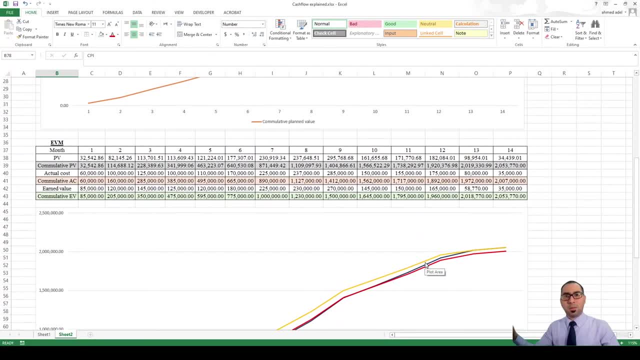 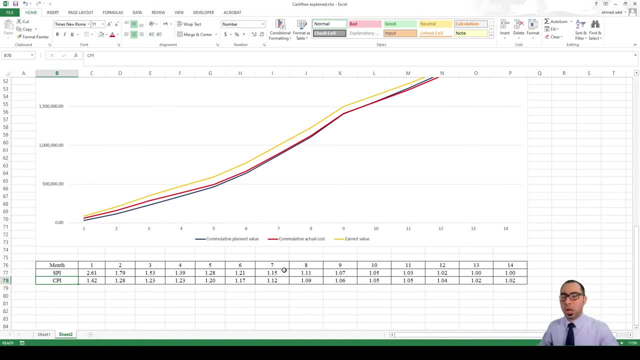 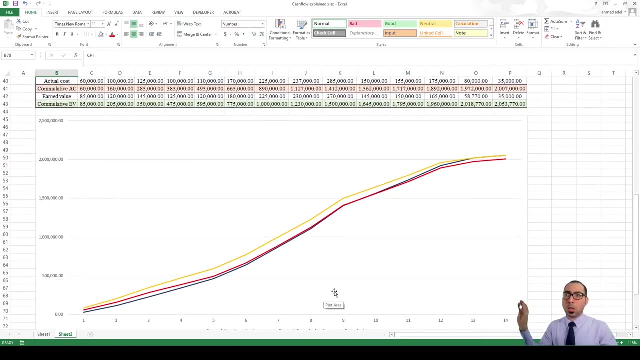 and guys, if any of you is planning to become a certified cost professional, the earned value management is a very big part, of course, plus many other knowledge areas, but the, the cost control and the end value management is one of the most important parts in the ccp or certified cost. 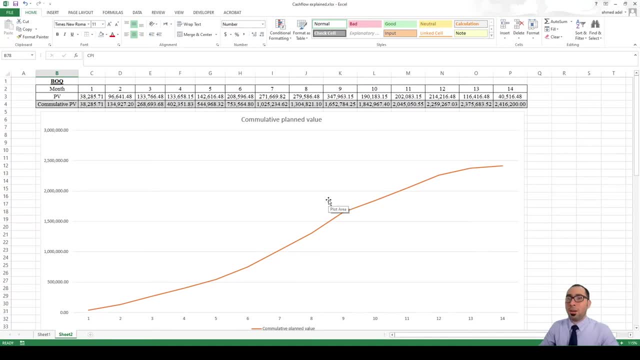 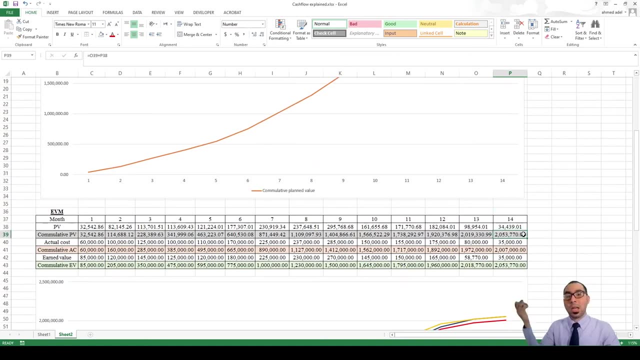 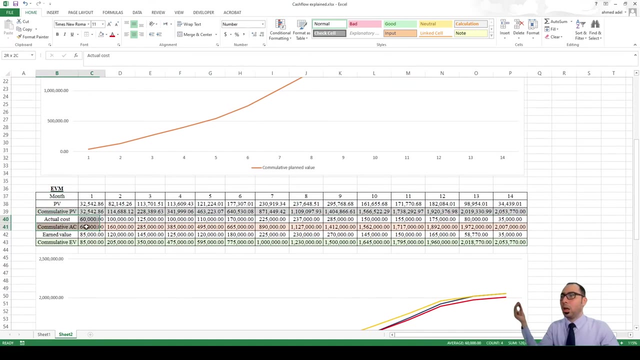 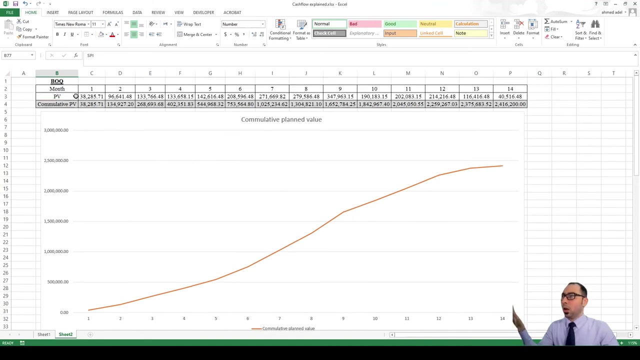 professional certificate and now you have the understanding. what is the boq? what is the difference between price and cost? let's say, or budget, okay, and only when you have the budget, okay, you can do that cost performance index and schedule performance index. guys, you can do here, because the 2.4, which 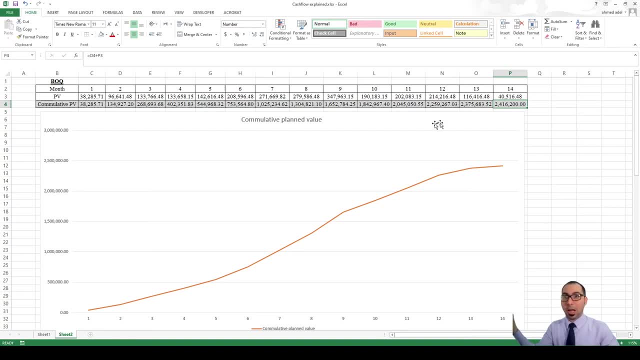 is the project value or project price that you have gave to your client. every month you will get the cost performance index, will see what is the worth of the like, what is the earned value, every month and you can get the schedule performance index to see if you are ahead of a. 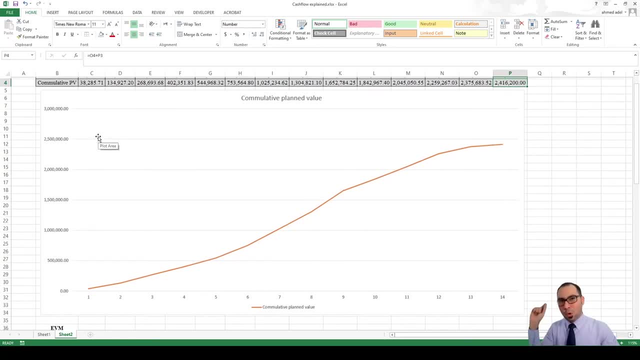 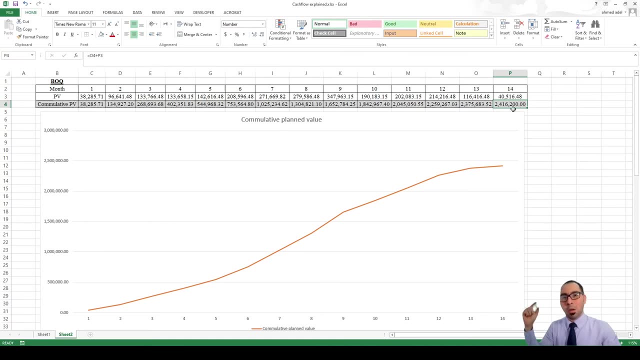 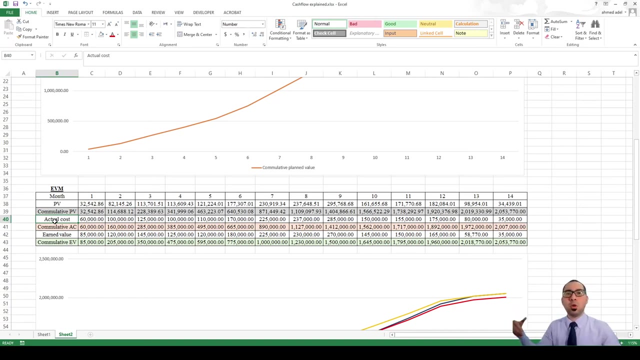 schedule or you are behind schedule. but if you want to measure the cost performance index also, you cannot do that on project BOQ because it includes margin. if you want to measure actual cost, it has to be against actual estimate, your budget okay. so it cannot be against estimate plus margins, which?